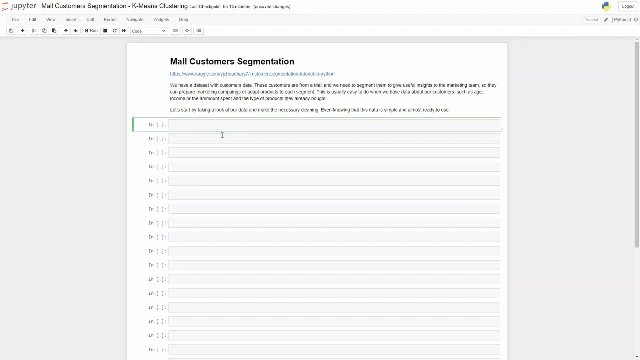 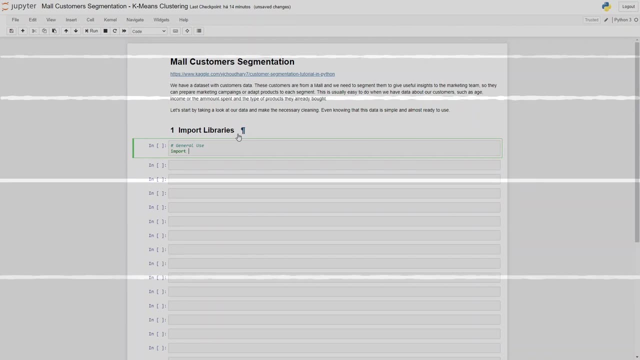 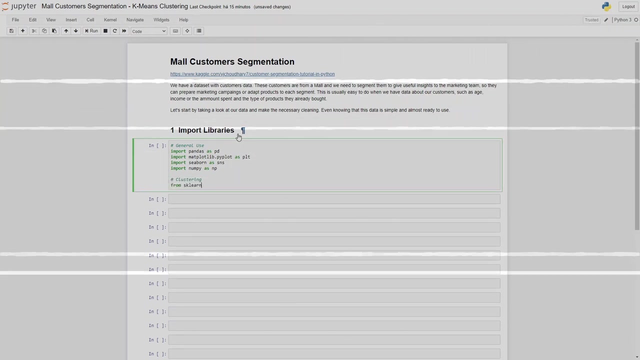 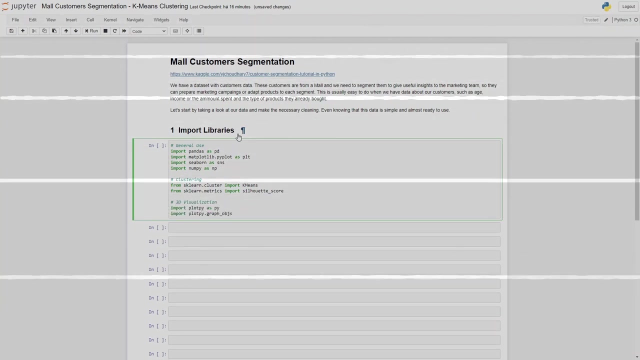 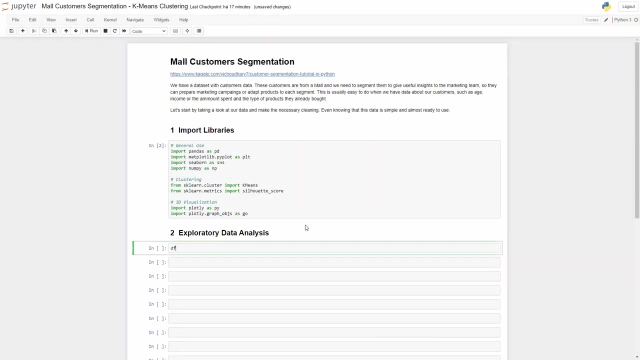 and let's start by taking a look at our data. so let's import our libraries. so so to start, this data frame is available in the link from the kegel. i will leave in the description and let's do pd dot, read csv to import our csv, and then the name of the csv. 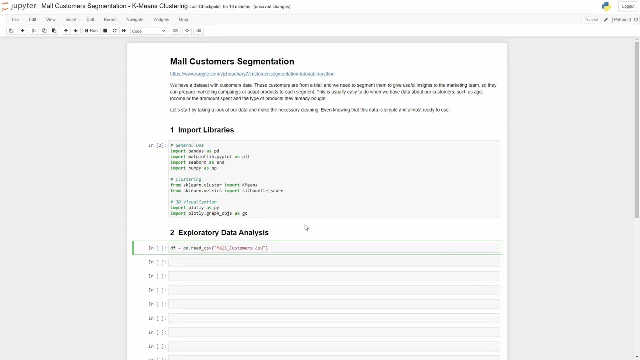 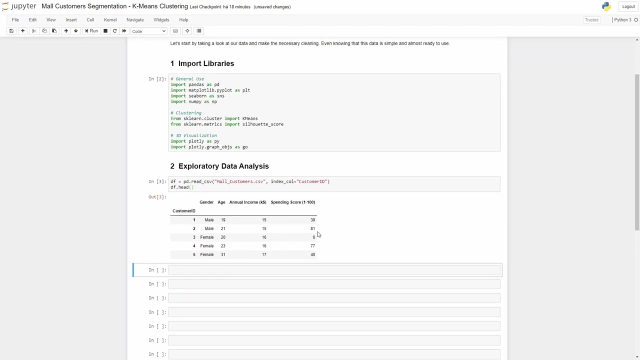 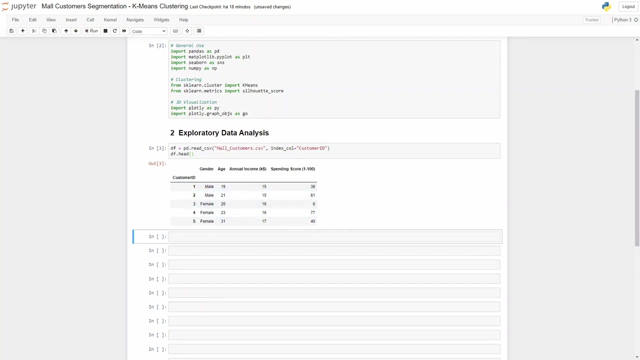 goes to mars dot, csv, and let's set the index with the customer id column. now let's see the head of our data set and, as you can see, we have custom id, the gender, age, annual income and spending score. so this is the data from our data set. and now statistics. 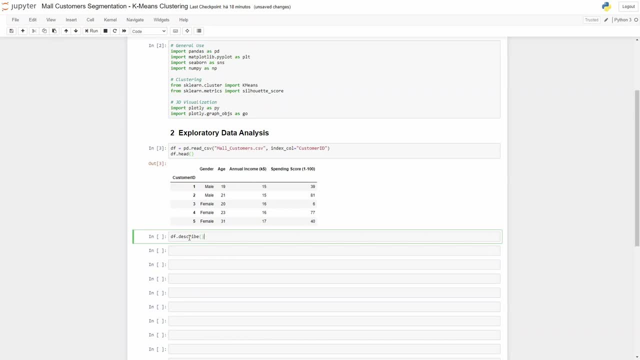 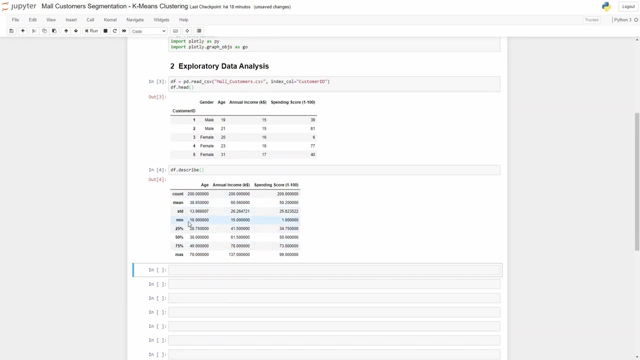 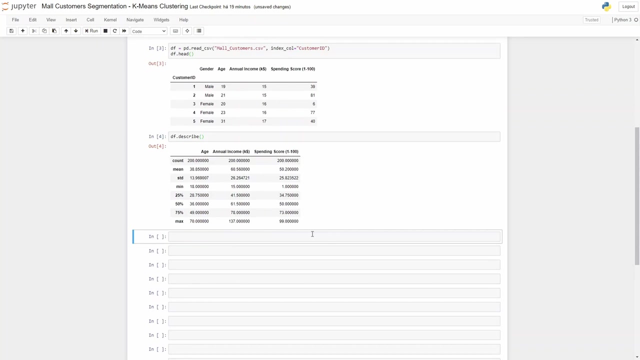 about our data set: describe. let's just describe to take a look at it. so we have 200 instance. okay, no negative values. it's okay in this column, the we don't have more than 100. max age is 70.. okay, i think there is nothing to do here. so let's see if we have 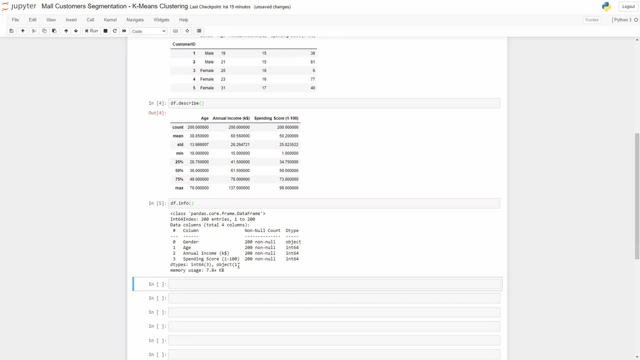 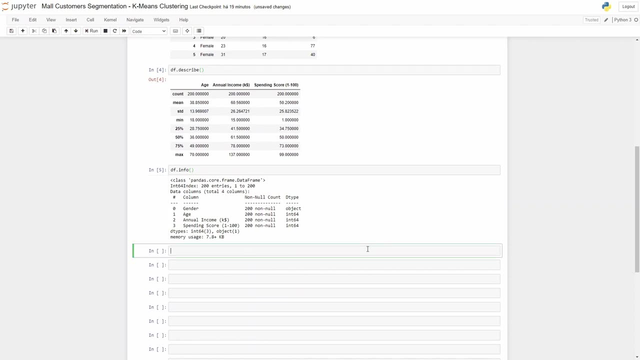 no values. no, we don't have no values, so that's great. we don't need to draw any instance now. one thing that we need to do is to drop the gender, and why? because we need to work with numerical data. so, columns, let's draw gender and don't forget, in place equals to true. 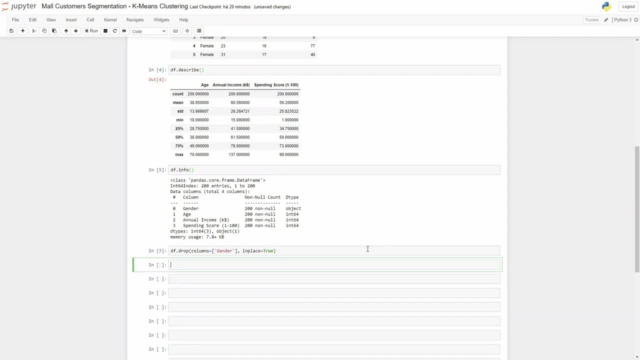 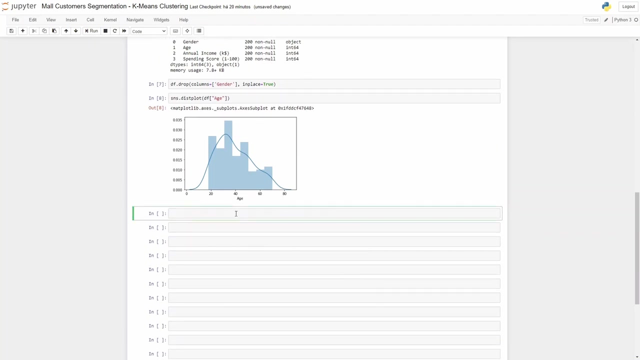 in place. it's an end, yeah, okay, now let's take a look at the distribution of our data. it is important to see if we need to do any transformation. i don't think so. h yeah, we don't have a great skewness, so let's do the same for the other columns for annual income. 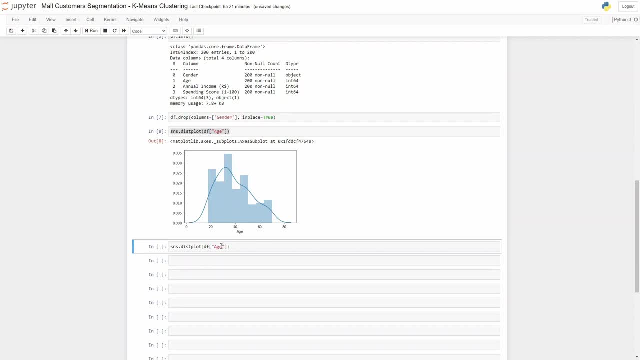 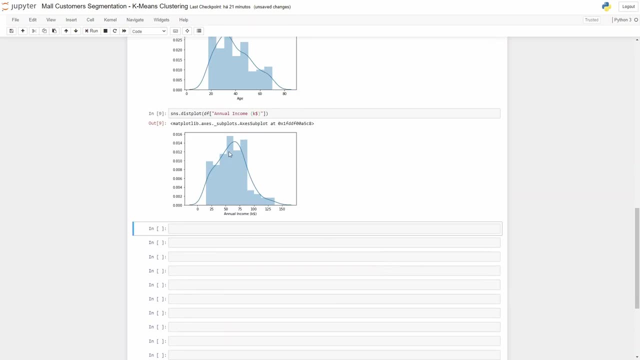 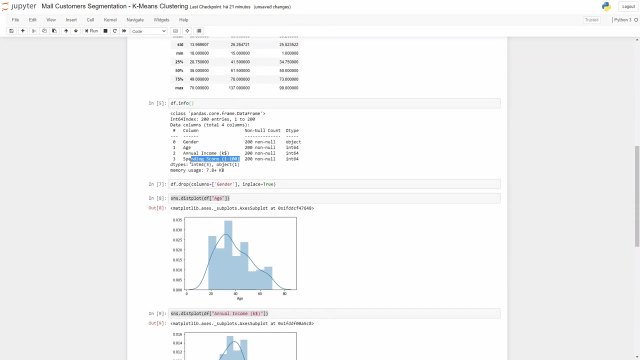 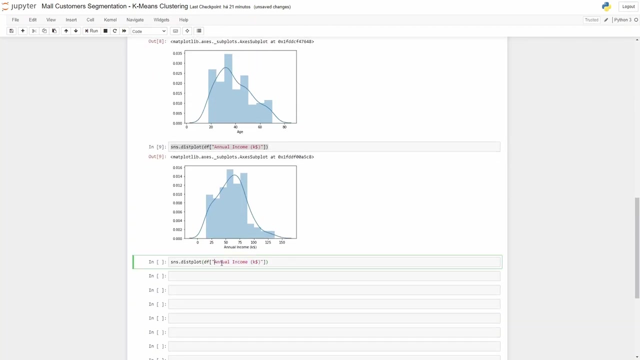 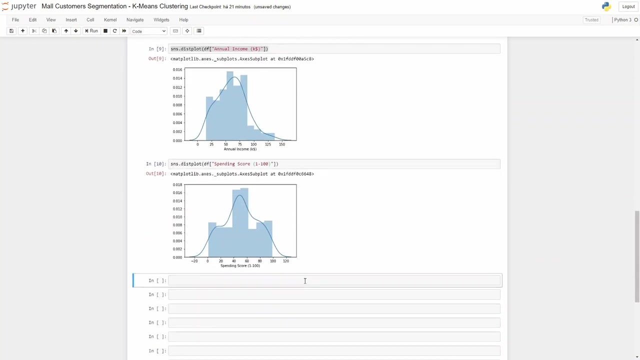 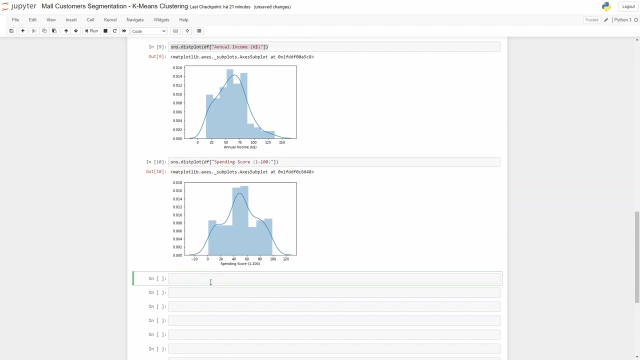 okay, it's not very skew, let's see, it's okay as well. so this won't be very significant for this won't be very significant for our model here, so there is no problem. so, and this one is great, yeah, okay, that's perfect. so now let's talk about the k-minus question. 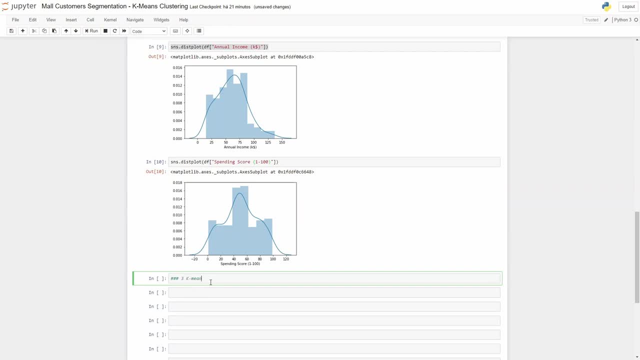 let me tell you a few details about this so you can understand it. it, The K-Means, is one of the most known algorithms to find clusters, works with large datasets while being very fast and efficient, and this technique was developed in 1957.. 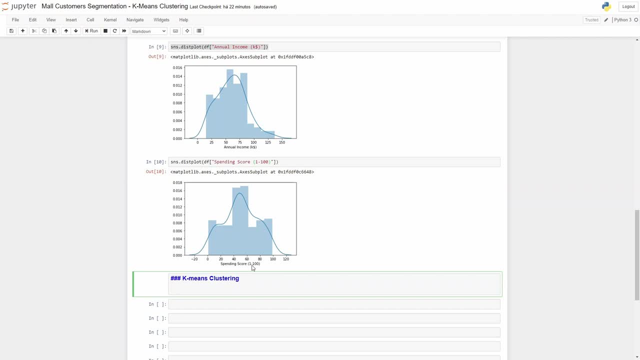 It is a centroid-based clustering algorithm. It tries to maximize the intra-cluster similarity and minimize the inter-cluster similarity. To start, we need to set the number of clusters for the K-Means algorithm, And how many clusters do we want? So we don't usually know this, but there is a way to try to find the optimal number of. 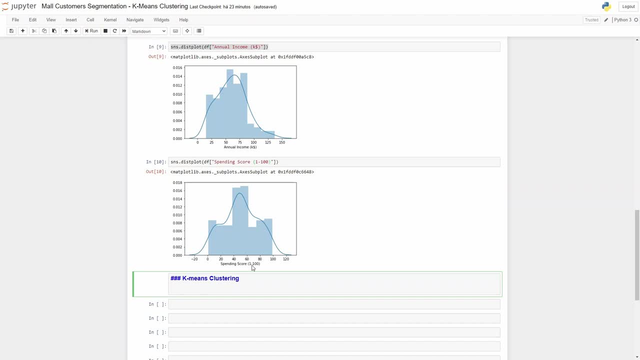 clusters. The algorithm will try to randomly select K centers, a number of clusters. These are called centroid. Then it will assign each instance to the closest centroid and calculate the centroids for each cluster form. Then it returns to the step 2., Which is assign each instance to the closest centroid. 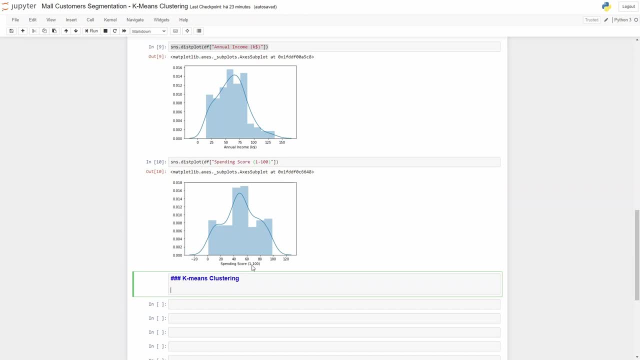 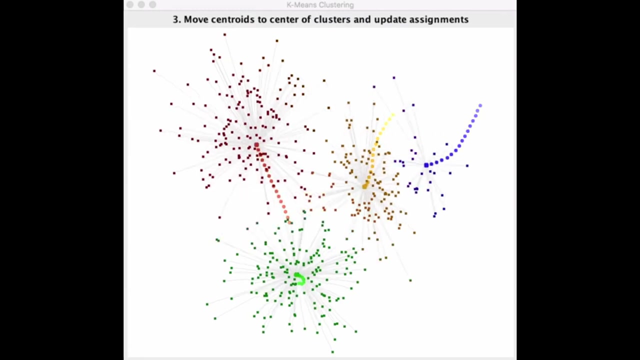 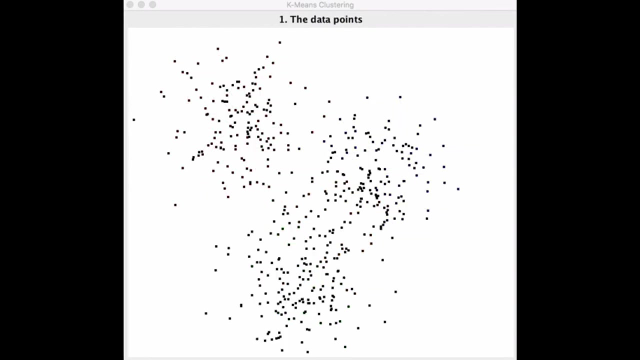 the closest centroid, calculate again the centroids and keeps doing this until the centroids don't move anymore. and so you can understand better what this means, i will show you this video. in this video you are able to see that we define the centroids, then we start moving and reassigning the instance until it reaches a stable solution. the centroid doesn't move anymore. 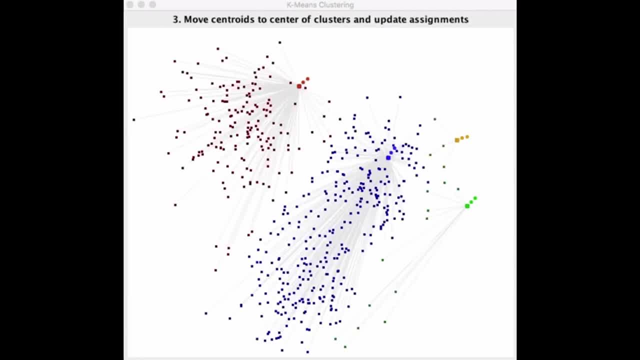 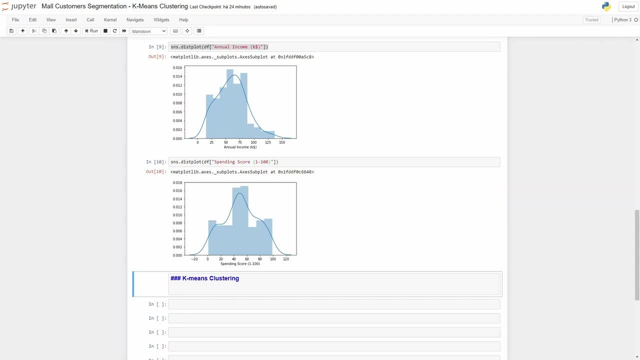 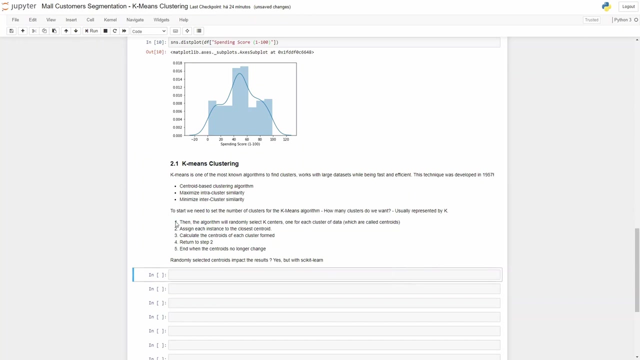 we can see another example. we calculate random centroids. they start moving and then it stops moving, and that's basically what we'll be doing here. so i will leave here an information. you will be able to find this jupiter notebook in the github repository. i will leave this and let's start by 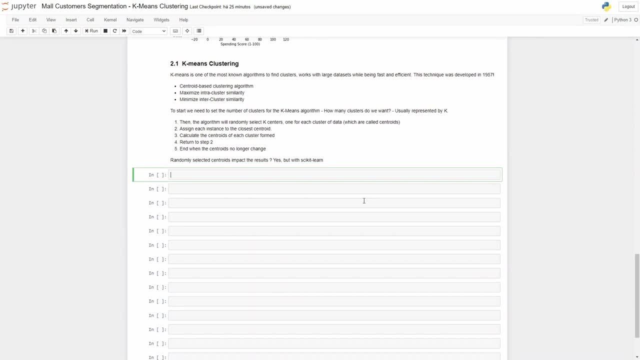 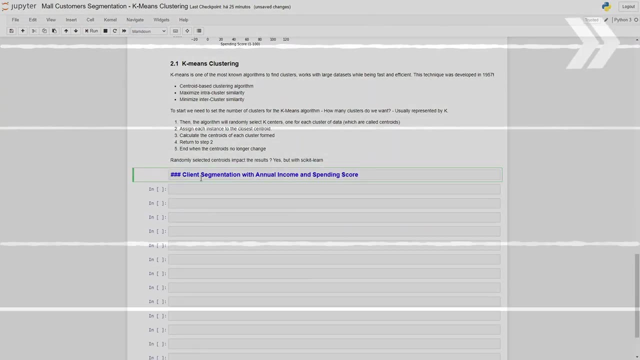 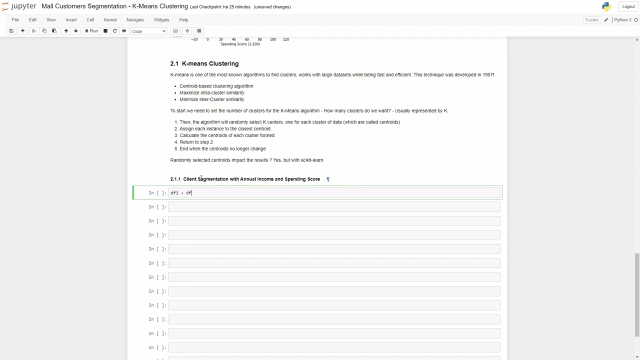 finding our approach: clusters, having in mind the annual income and spending score. now let's define a new data frame with these variables. you can calculate these with whatever variables you want. so for this purpose, i will start with these two and then we'll do another one for all the variables. 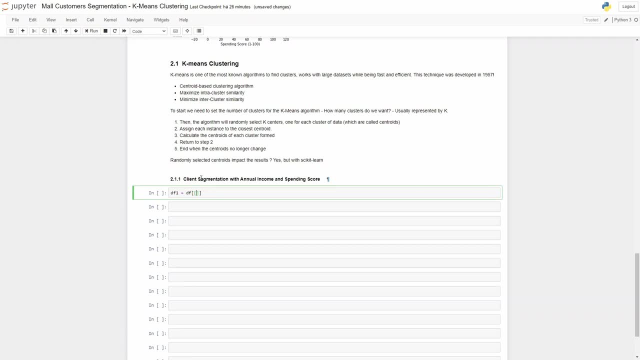 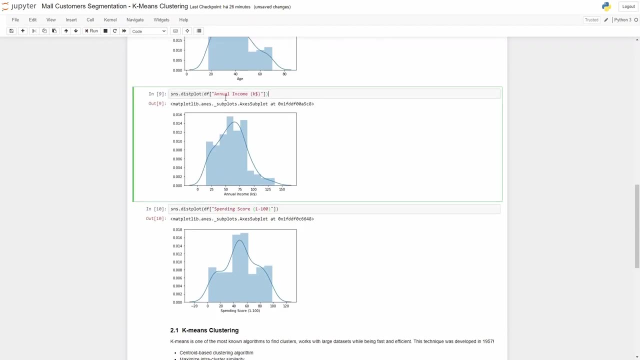 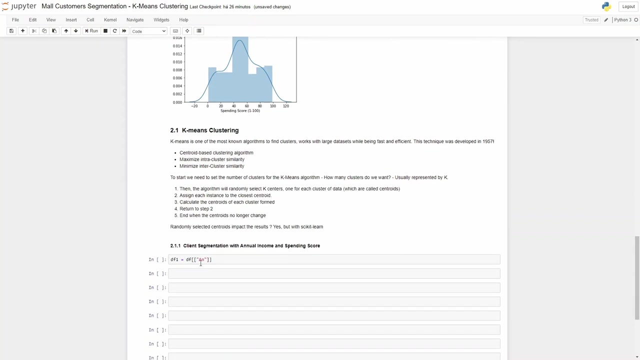 and that's it for this video. thank you for watching and see you in the next video. bye, bye will teach you how can you do a 3d plot, the frame. so it's more easy if i copy this: one annual income. if you want to practice, you can try to change the names of these columns, because 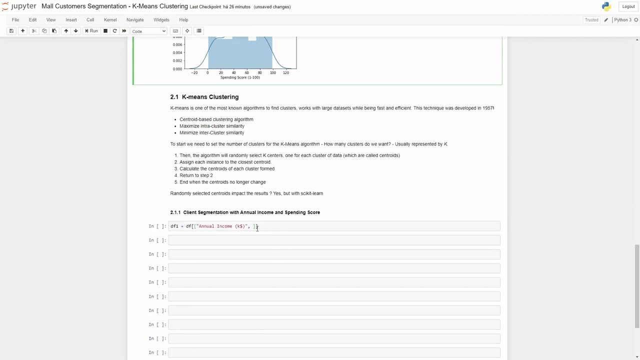 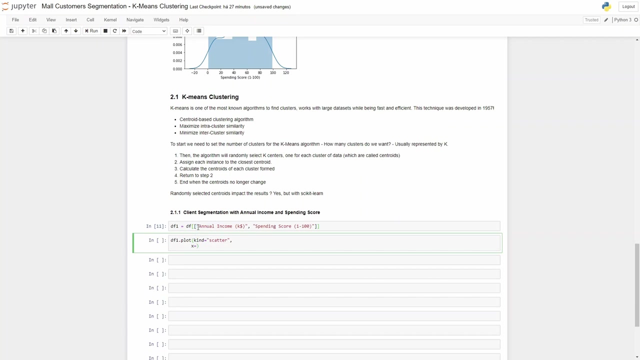 there is no need to have this huge name. it's bittersweet. so this is our dataset, and let's visualize our data. maybe we have enough feeling for it. we can choose a kind of scatterplot, and then let's define our x, which is the annual income. 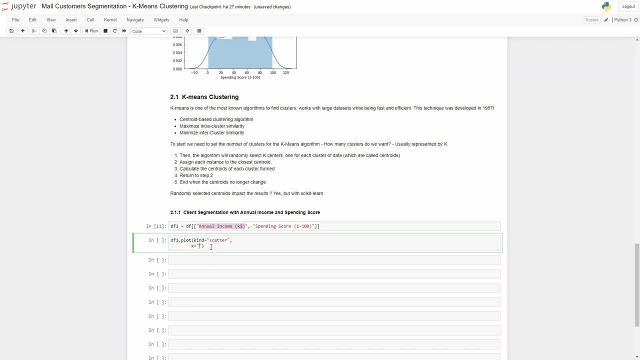 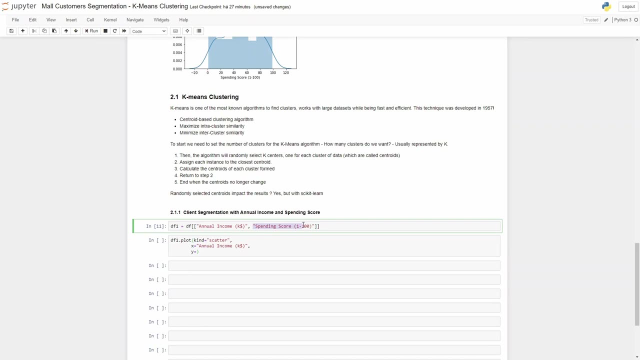 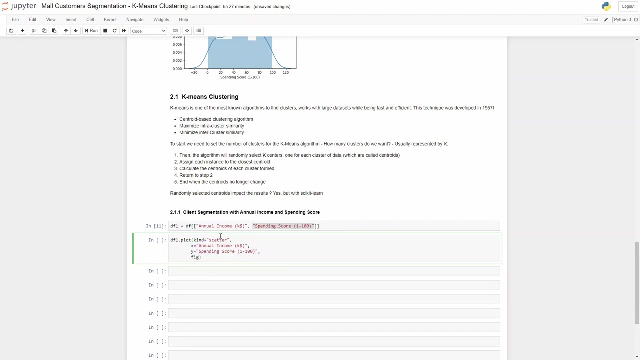 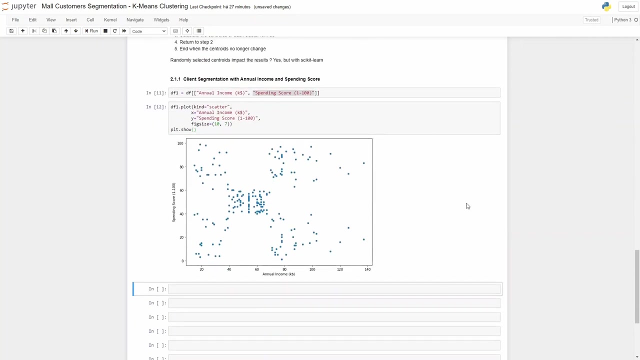 income, then define Y, which is the spending score, and then we can do: fix size equals to, let's say, 10 by 7. no guilty show, we are ready. so this is our data and you probably are able to see how many clusters you may have here. how. 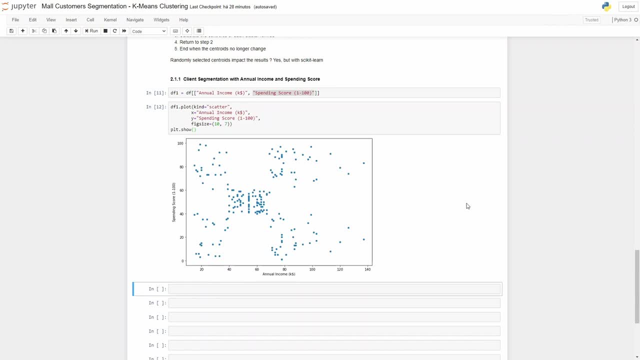 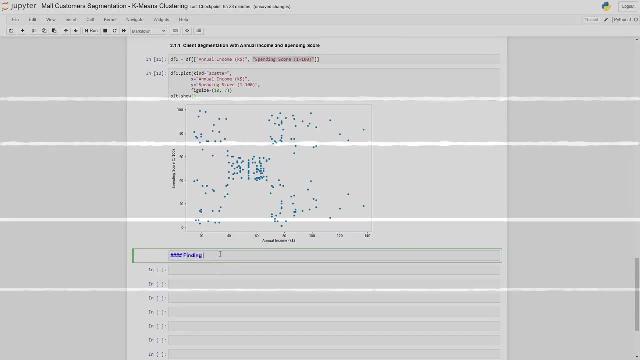 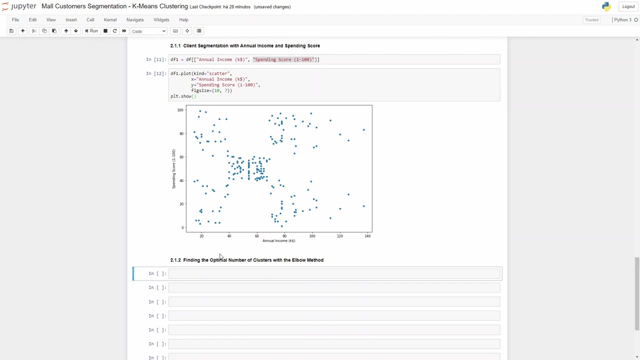 many clusters do you think we have here? okay, let's use a way to find these clusters, which is with the elbow method. this is one of the limitations for this kind of problems. we need to set the initial number of clusters and most of the times we don't know. we have no idea. 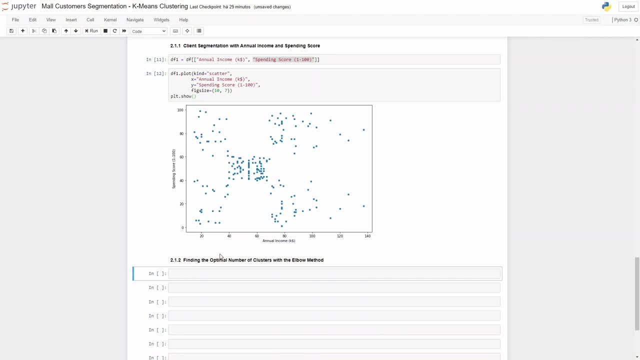 and to try to understand that we can use the elbow method to find it. the elbow method is built with the inertia from each number of clusters, and the more clusters we have, the closest each instance will be to the central right. so we have more centroid, so each point will be closer to the centroid. 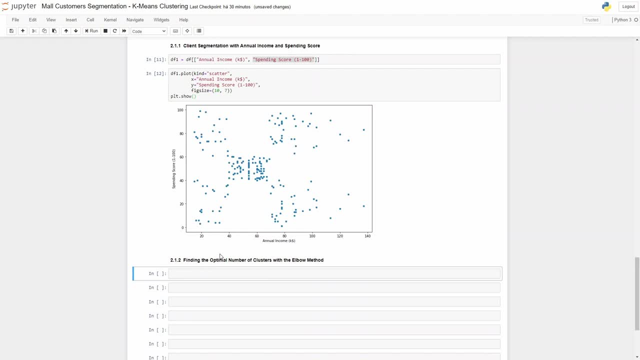 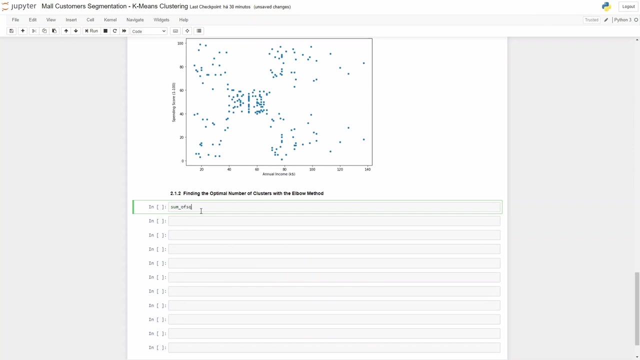 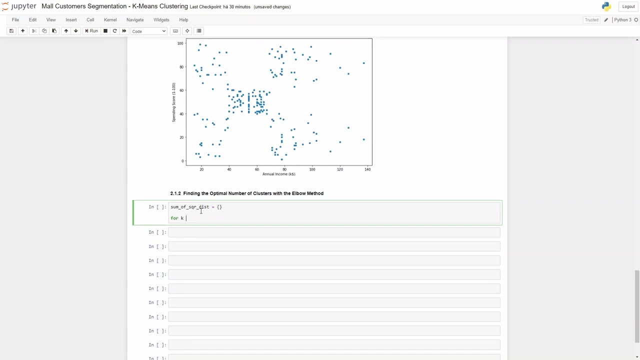 right, which can be represented by inertia, and that's what we are plotting here- which will be decreasing while the number of clusters increases. let's compute that. so let's build a dictionary for the sum of square distance and then let's do a loop for each K, in range of 1 to 10, for example. this is: 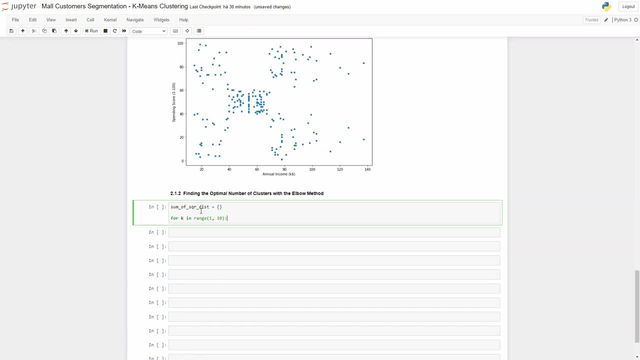 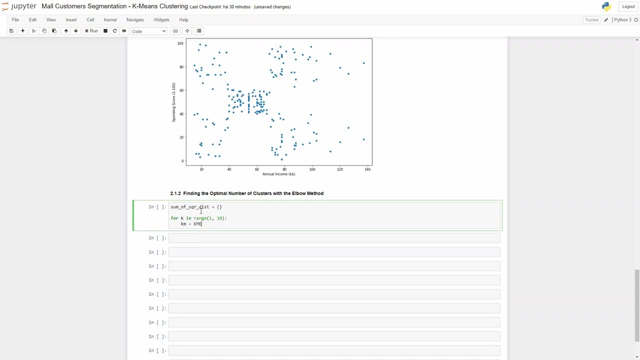 the number of clusters where you will be doing this, let's use key M, for key means equals to, and now we call the k-means from the scikit-learn library and define the n clusters equals to k, and then we'll use the init, which is an initialization method for the centroids. 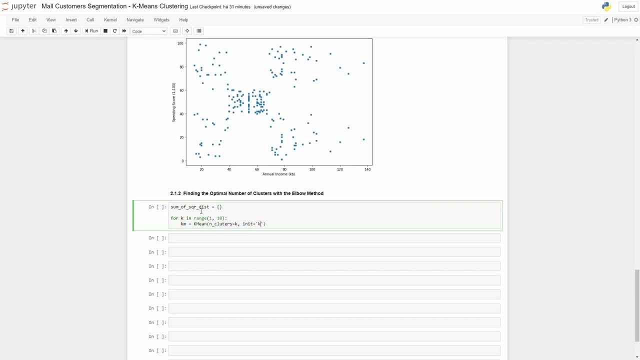 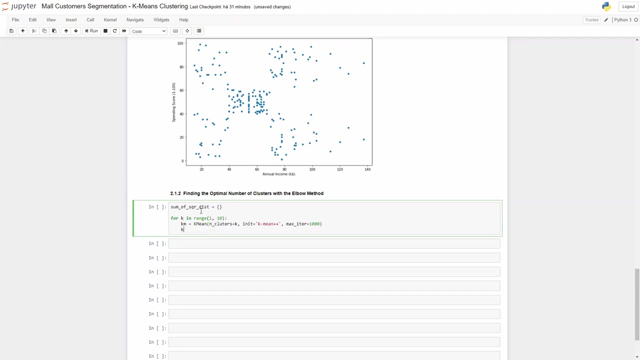 and in this case we'll use the k means plus plus, which is fair apps, the best way to initialize our clusters. i will leave also a documentation about this so you can understand better. and then the number of max iterations, let's say 1000. so, and now we will fit our k means into our data frame. and then let's: 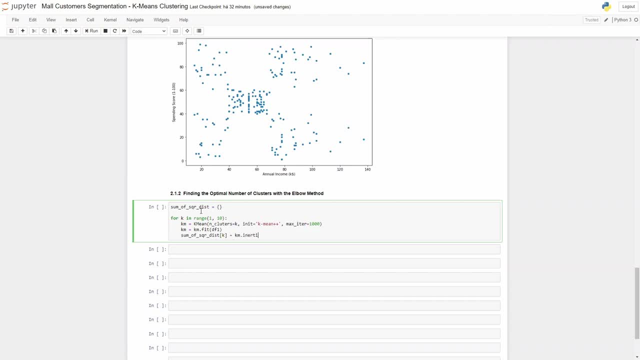 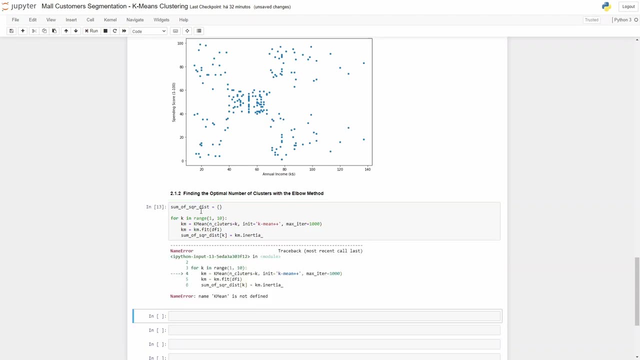 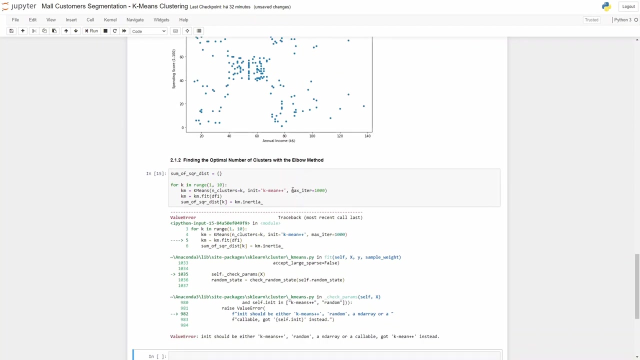 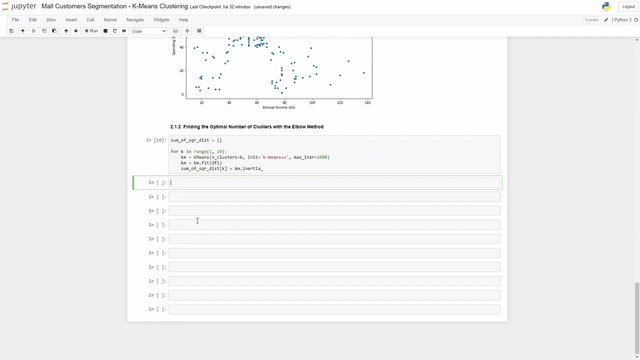 save it. and now let's save our inertia. for each k means okay. you can mean this is not defined. of course it's not. it's missing an s clusters, so many errors. what's going on? all right, now, it is right. okay, now let's do a plot to visualize our elbow method. so i said, yes, let's do a point. 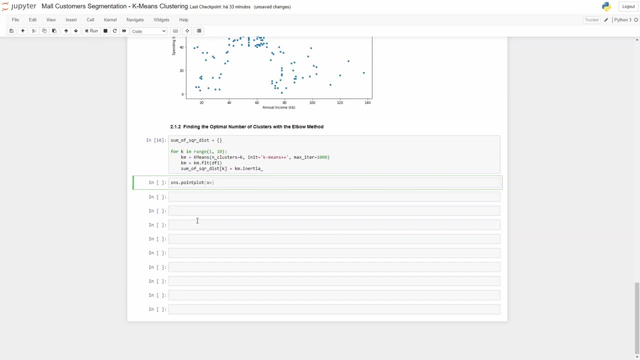 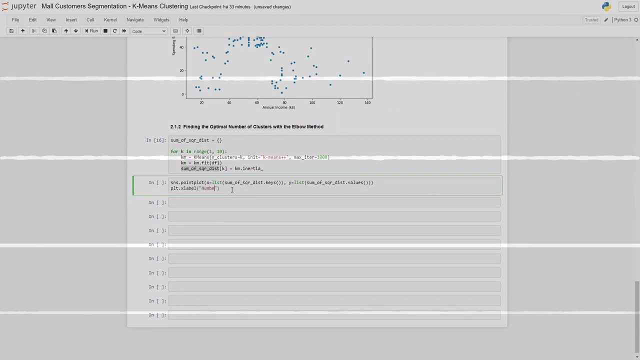 plot. and for our x, we will use a list for our- let me copy this- key values. and then let's do the same for our y, which is equal to a list for the sum of square distance for the values. okay, and now let me just plot labels. 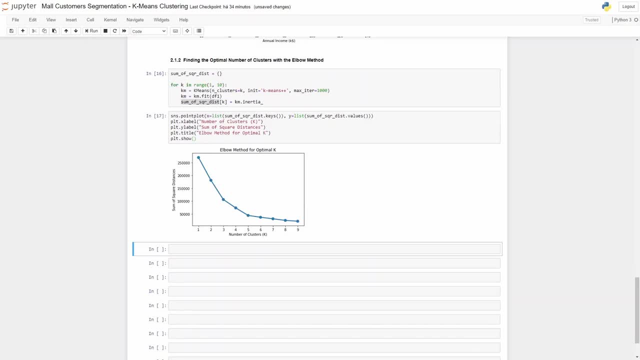 okay, here is our plot to display the elevation. so we will just plot labels, the values which are called the upper and the lower top left side of the circle. so i'm just going to plot the top left side of the circle, okay, so here is our plot to display the elevation. so we 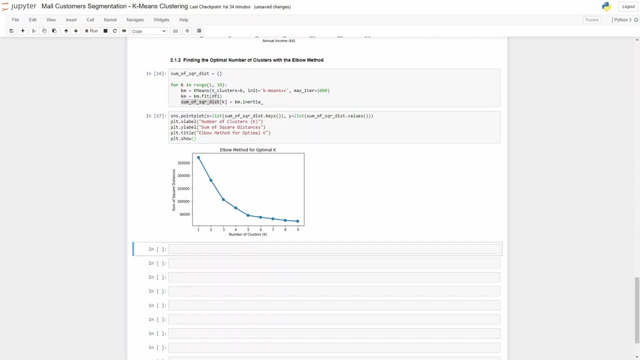 method and if we look at the elbow in this plot, we are able to observe that inertia stops decreasing significantly at k equals 5 after that point. usually more clusters doesn't give you much more useful information, but as a data scientist you will need to interpret the business context and the marketing. 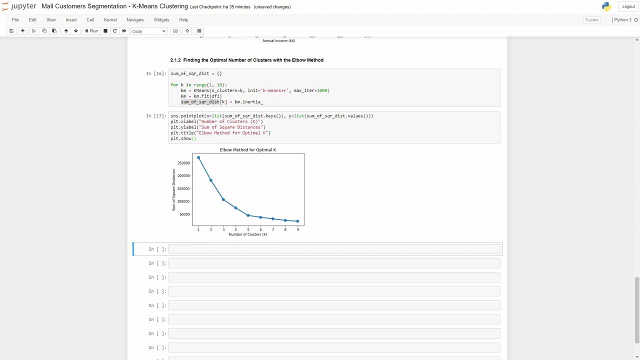 objects. does it make sense to have more clusters? does it make sense to have fewer clusters? but we'll stick with this one. let's continue, because there is also another way to help us defining the optimal okay- the number of clusters. I'll use it at the end of this as a metric to evaluate our decision. so for now, let's. 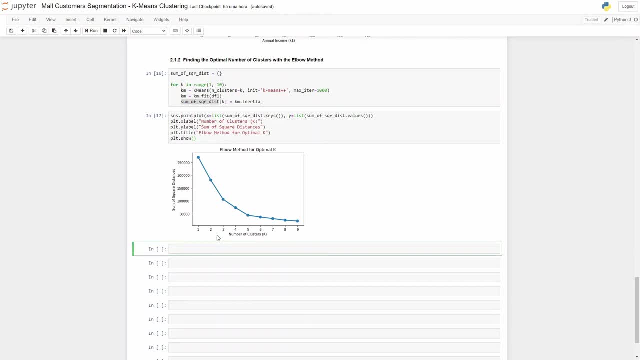 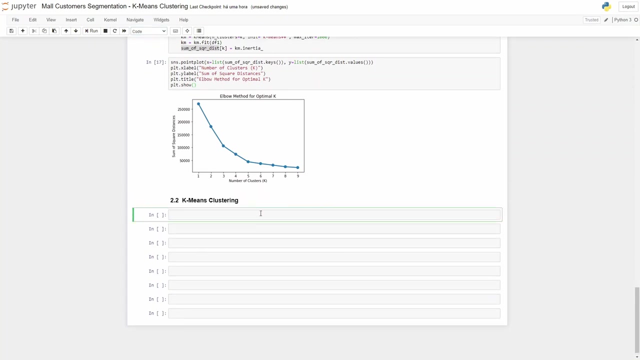 keep k equals to 5. so now let's do the k-means question, now that we find out the optimal, okay, the k-means is very sensitive to the initial positions of the centroids as well as the existence of outliers. so far we can tell that we don't have outliers from the distribution plots, but there is. 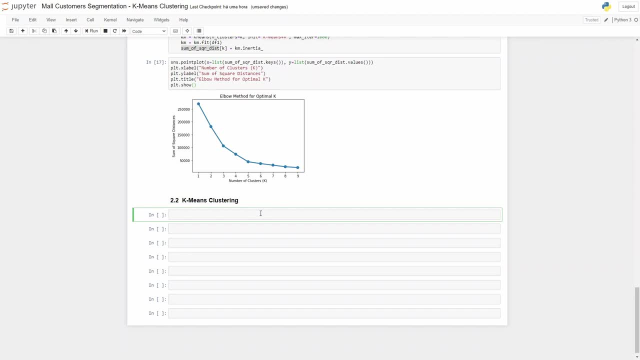 a way that k-means was improved for the initial position of the seeds, which was true, the k-means plus plus initialization. I'll leave the link to below with the article so you can read more about it. let's start by creating the model for our k-means with n clusters equals to 5, and then the init. 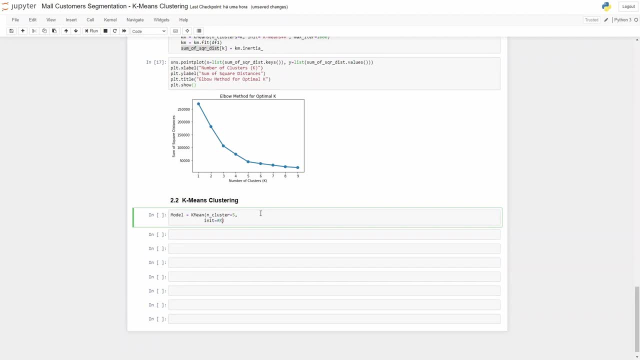 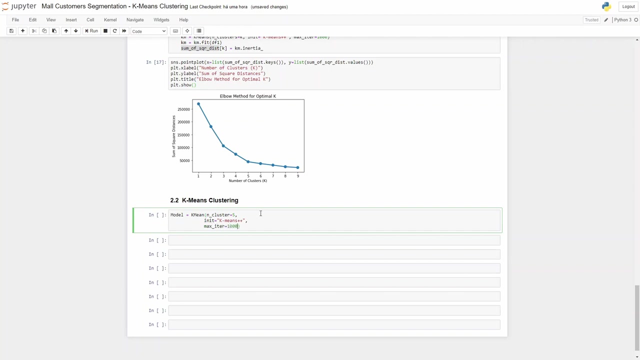 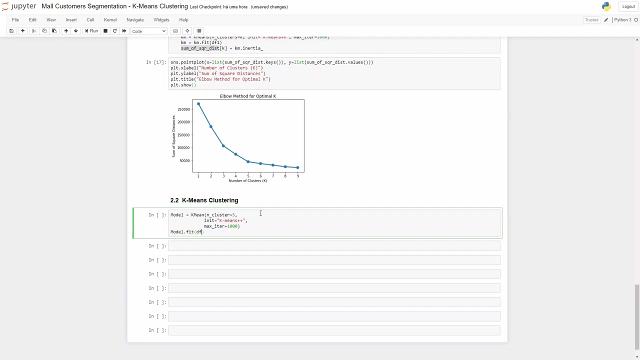 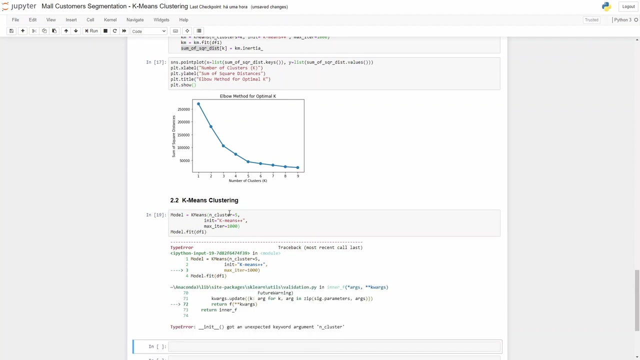 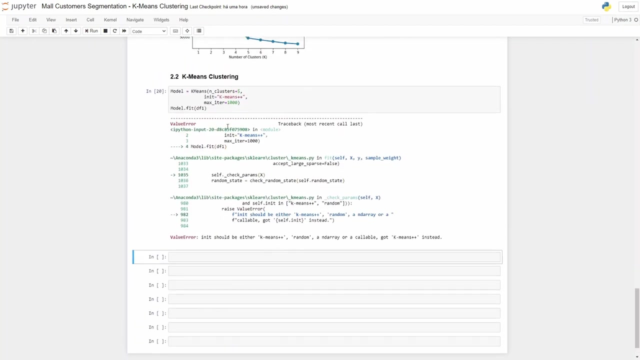 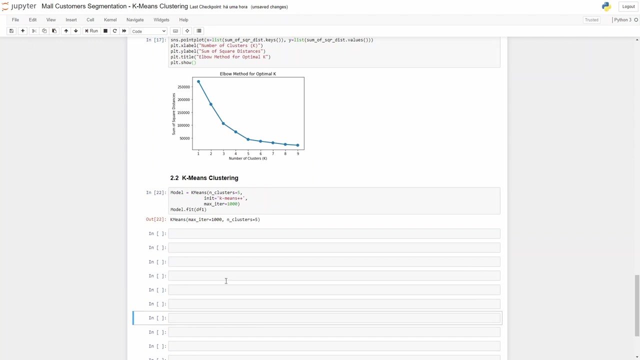 will use the k-means plus plus, and the max number of iterations equals to 1000. and then we use modelfit with the data set that we want, and again, I'm always forgetting the s in both places. and now, all right. and now what can we do with this? so we can print, for example, our 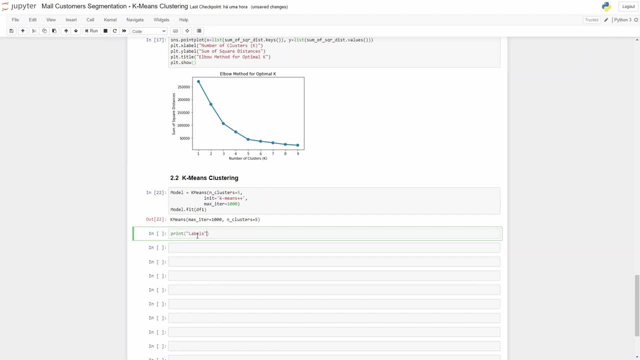 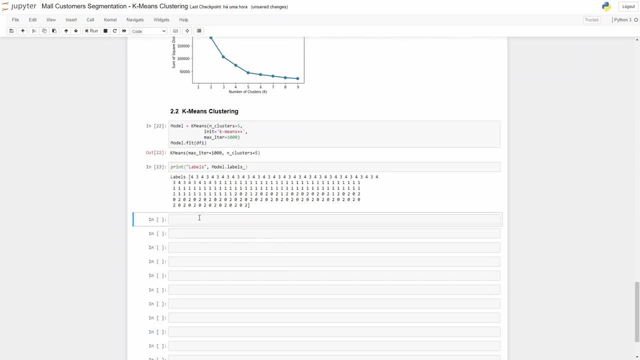 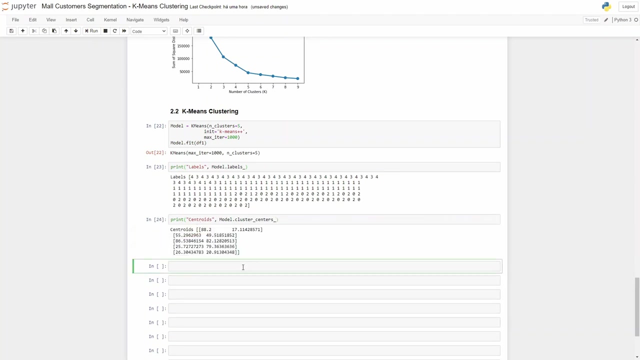 labels which are the clusters. so for that we use modellabels underscore, and these are the labels for from our model and we can also print our centroids. we use modelclustercenters, so for that we can also do the centroids and assign it to the modelclustercenters. 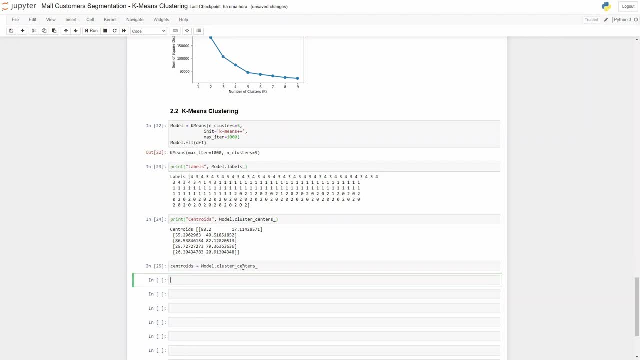 so we can save our centroids. and now we need to assign our clusters, our labels, to a new data set. for that let's do: def1 cluster equals to def1.copy, and then def1 cluster. and now let's create a column called clusters, our cluster with 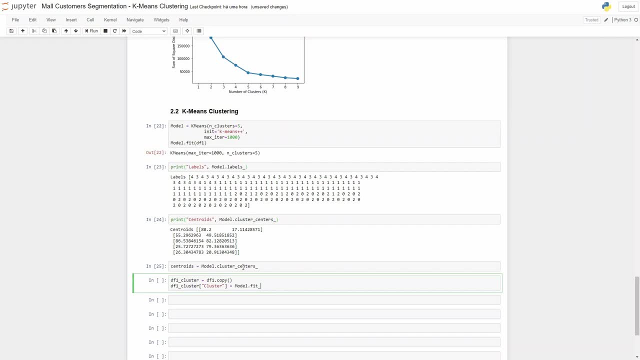 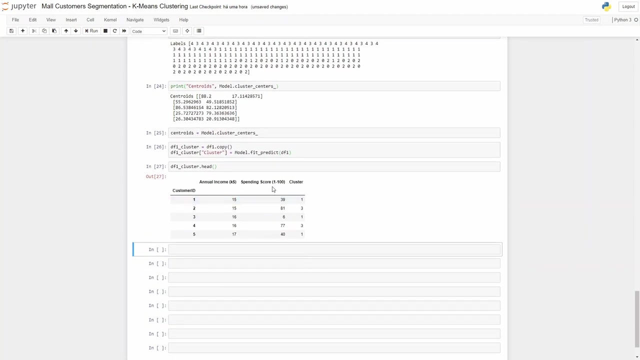 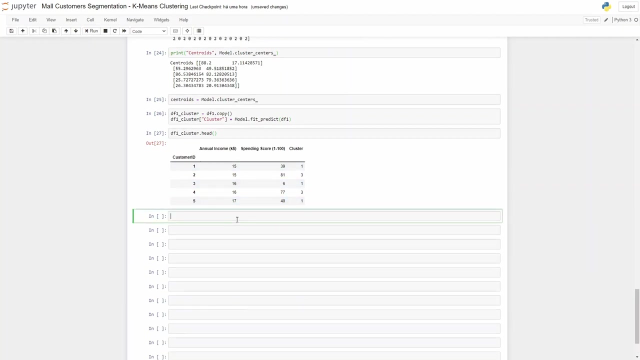 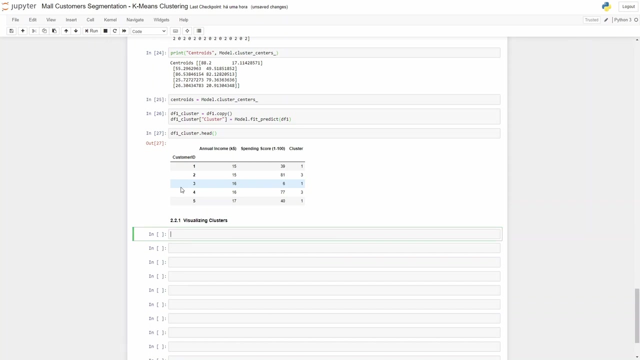 modelfit predict the f1. okay, and now we can visualize our data set head. so, and now we have annual income spending score and the cluster which instance is assigned to it. now, to visualize our cluster, let's do the visualization. let's first create the colors that we will be using. 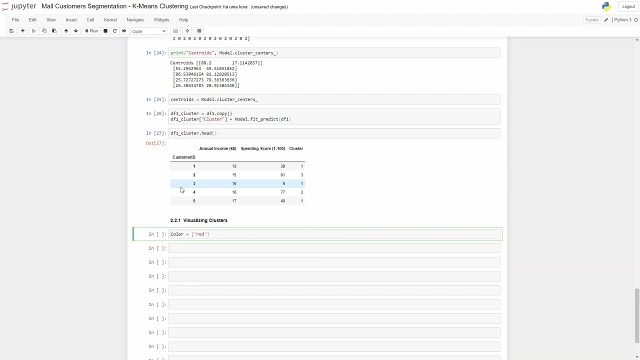 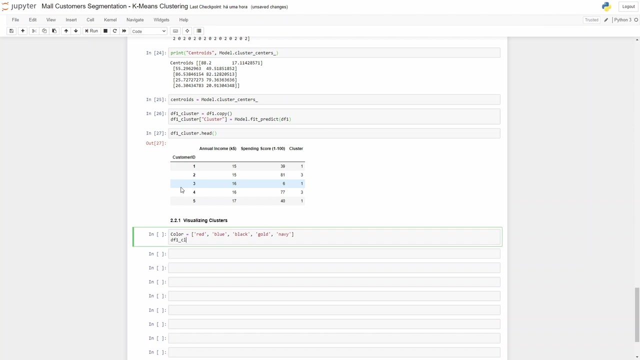 you can use any colors you want. so let's for example, red, blue, black, gold, and it can be blue, brown, right. so, and now we, we will assign to a new column these colors, and for that we'll use the map function. so f1, cluster and then assign to the cluster. 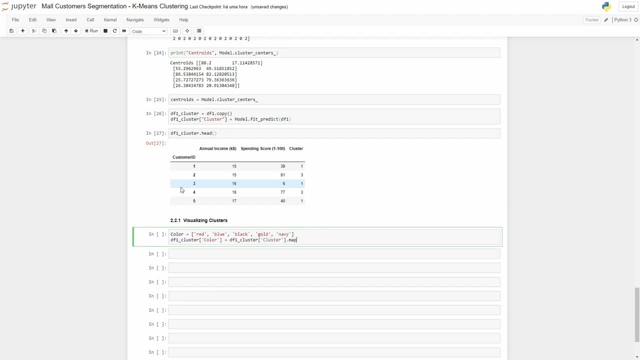 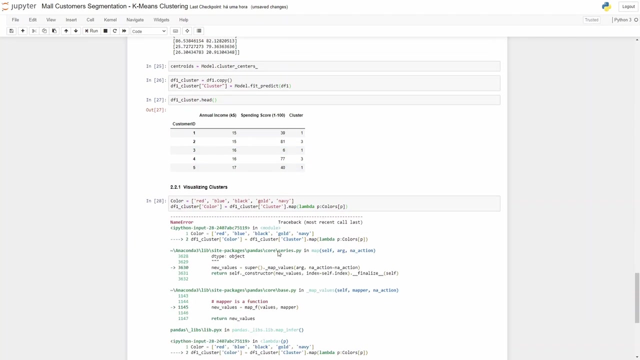 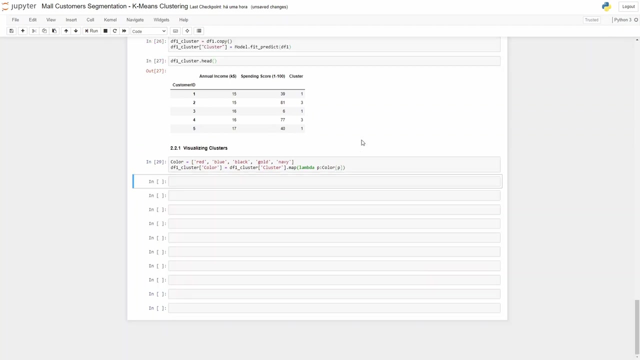 column dot map and now lambda p for colors p and this should do the work. what's wrong here? color is not defined. okay, yeah, of course. and now let's plot our clusters and centroids. to do that, let's plot a figure: fixed size equals to 2010. now reality, let's do. 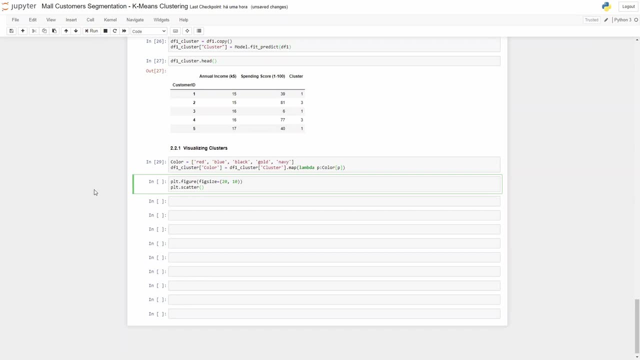 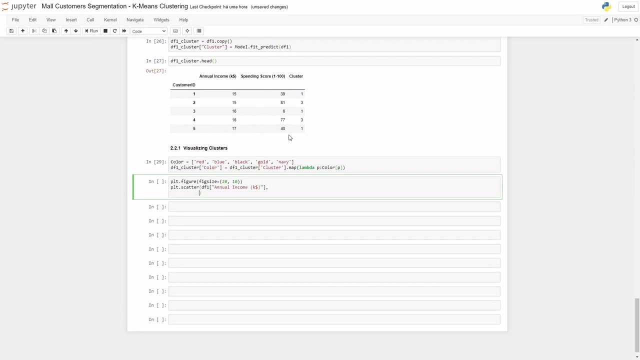 work. and now lambda p for colors p, and this should do the work. what's wrong here? what's wrong here? let's do a scatter plot for def1. let's call the annual income column our values. let's do the same for def1 and spending score values. 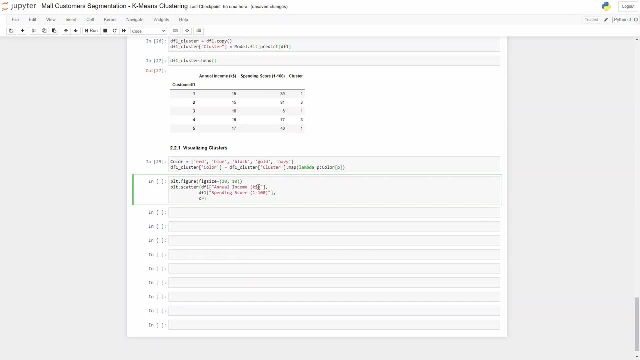 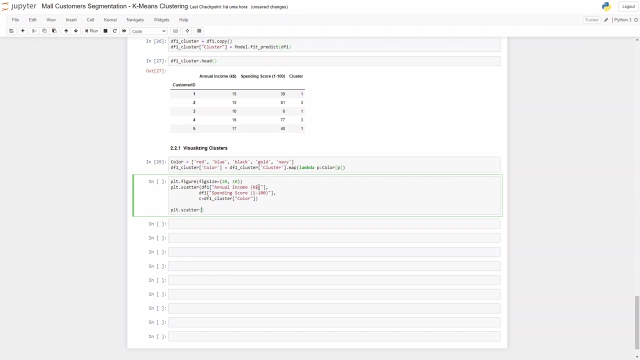 and now let's assign the values of the values of the cluster and let's call the annual income column for the values of the cluster and let's call the annual income column colors that we defined. Let's also do a scatterplot for the centroid, So let's 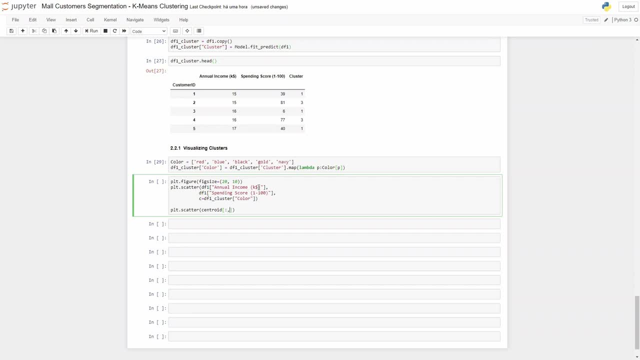 define the X centroid and then the Y, And let's assign a color for the centroid. It should be different from the ones that we already used. It can be green. We didn't use green. And the size of these dots? Let's put this value, for example. Something is wrong here. This one. Okay, Now we 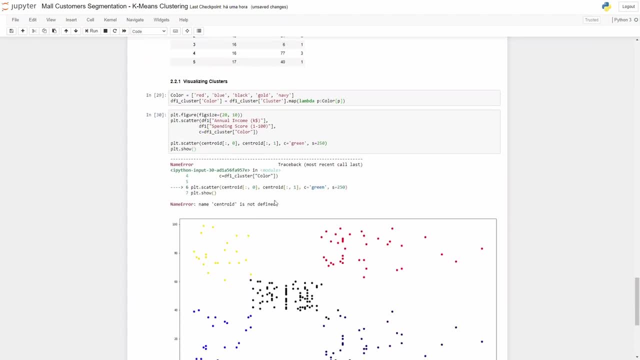 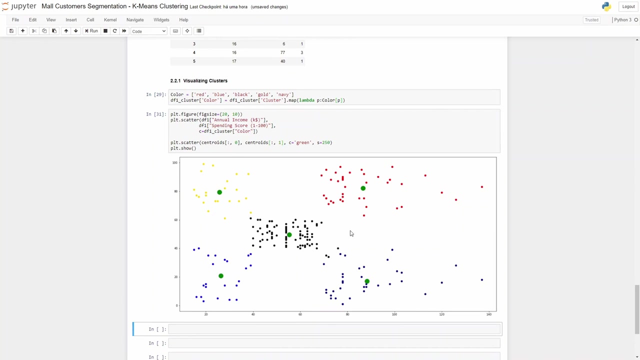 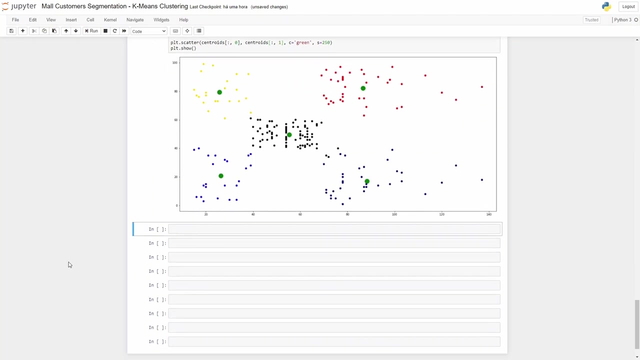 got this show And we should be able to see: Yeah, It's missing an S. I don't know what's going on today, Missing a lot of S's. And here is our five clusters, with the five centroid With different colors assigned to each other. We already did the clustering, Now we need to. 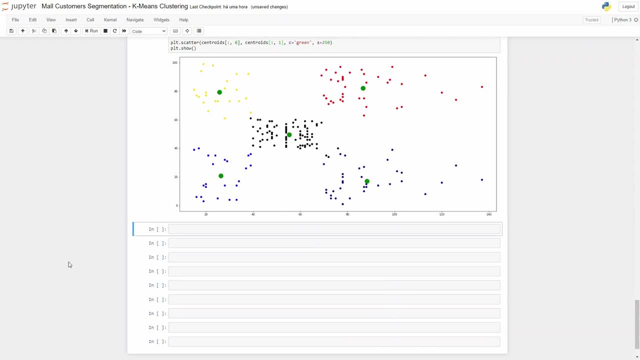 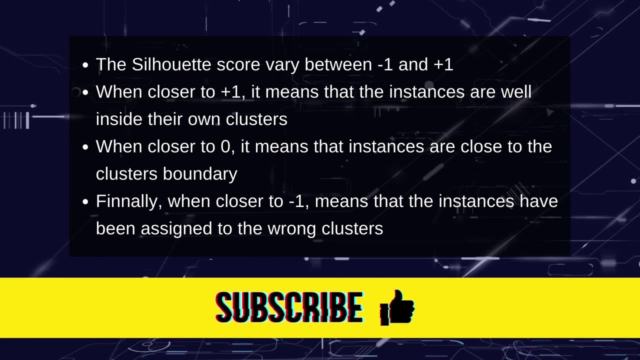 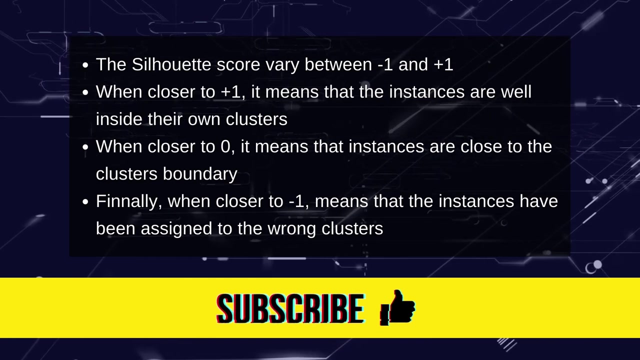 evaluate our clustering And, as I said here earlier, We can use the seed weight score. And the seed weight score varies between minus one and one, And the score closer to plus one Means that the instance are well inside its own clusters, And closer to minus one It means that instance 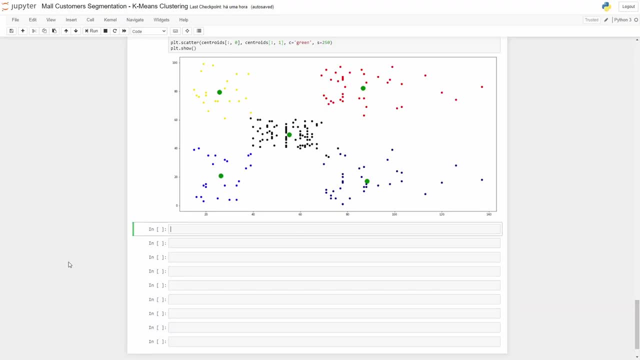 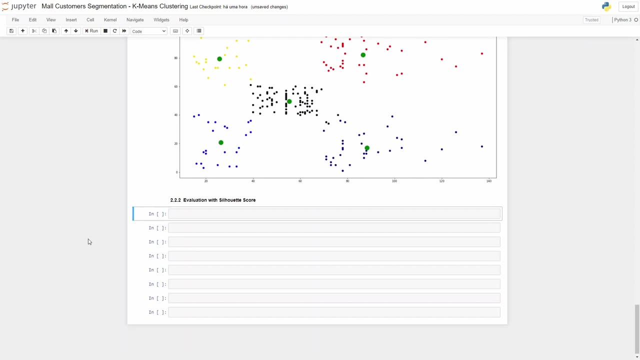 have been assigned to the wrong clusters. So let's see how can we do this. So usually the seed weight score is more precise than the elbow method. However, it requires a lot more of computer power. So we need to define a labels variable, And that's easy. We just need to call the model. 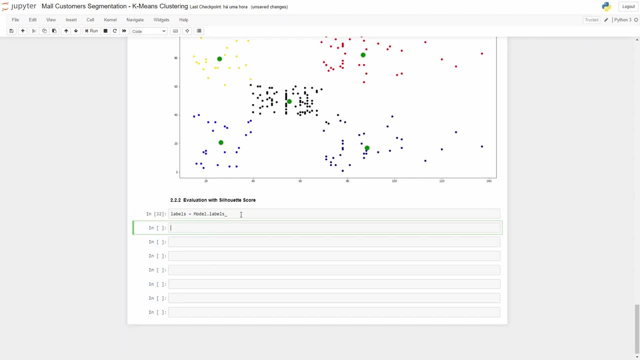 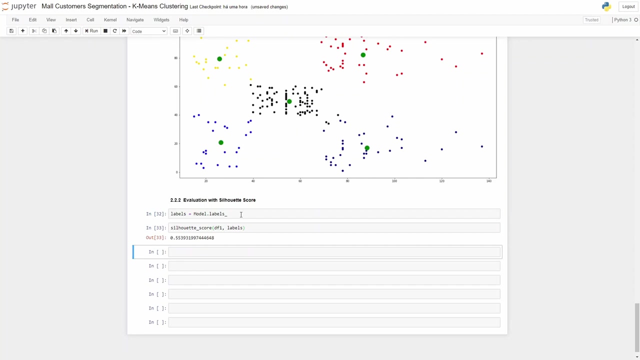 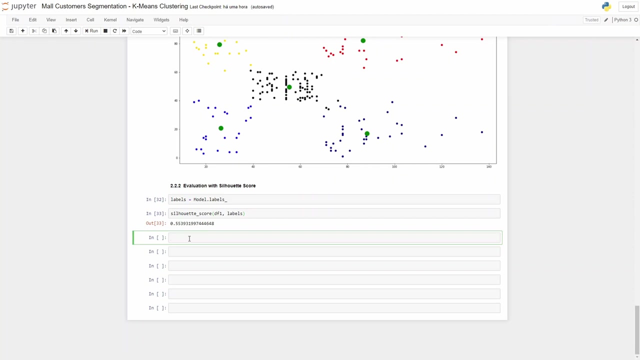 dot labels underscore And after that we will use the seed weight score And call our df And our labels And we have the score of 0.55.. And now we need to compute each seed weight score for each k And after that we will be able to see. 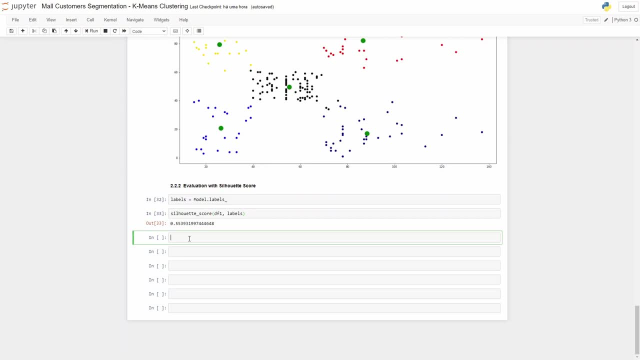 if we choose the, And for that we will use code similar to the elbow method. Let's define a dictionary To store our seed weight scores And for each k In range From two To weight, for example, We will compute: key m equals to the key means With n, cluster equals to k. 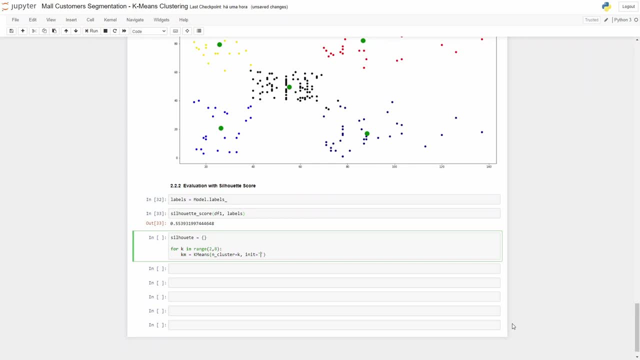 The init equals to k means- I won't wrong this one again- And max iterations equals to 1000.. Now k m dot fit With df one And see the way Of k equals to see the weight Score Of df one And k m dot labels. 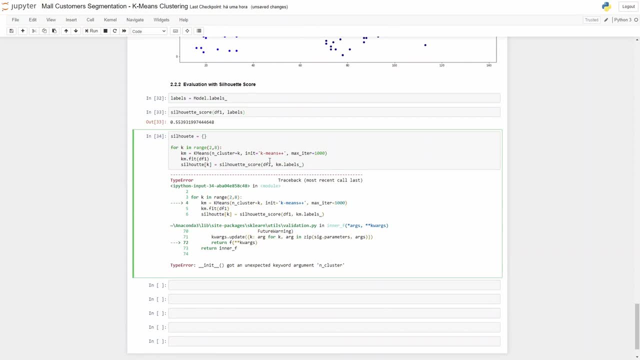 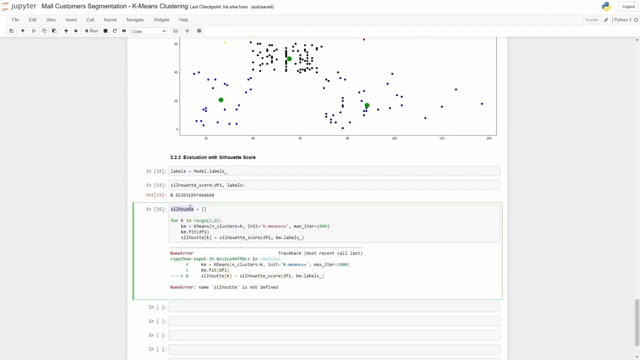 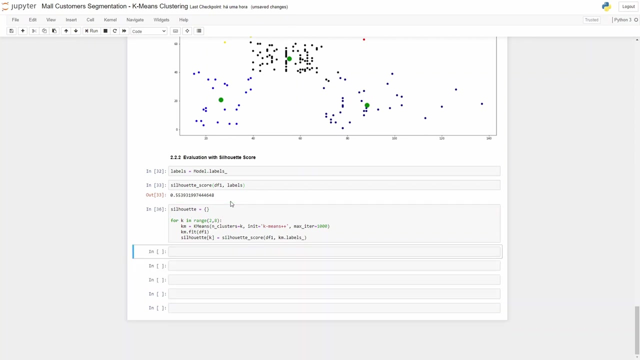 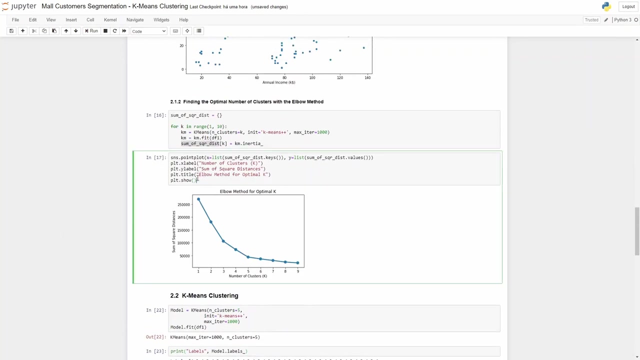 Okay, Another error. Ah Yeah, I didn't miss initialization, But missed the clusters. Seed weight is not defined, So this is wrong. Okay, Now it is, So Let's grab the code from here. It is pretty much the same, We just need to change a few things. 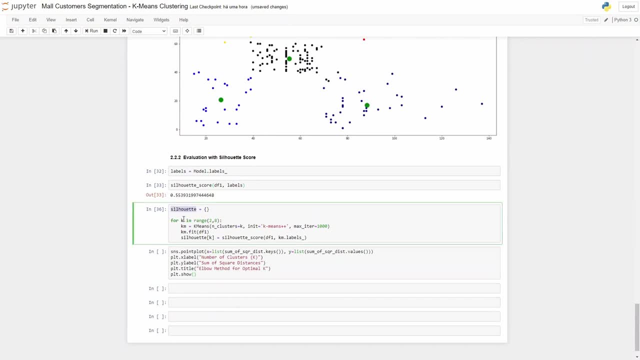 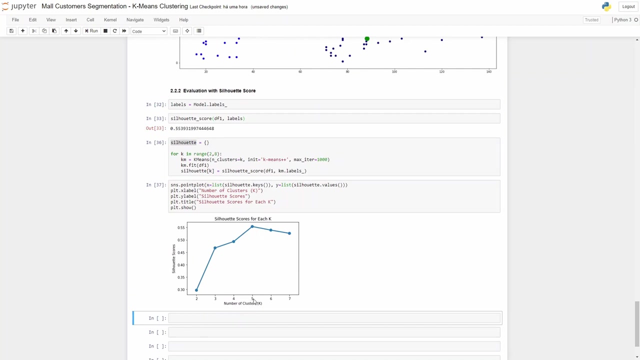 So We will need this dictionary, The seed weight, And now we will need Seed weights, Scores, Number of clusters And here is silhouette scores for each key. So, as you can see, the best silhouette score is really 5k, which confirms that we choose. 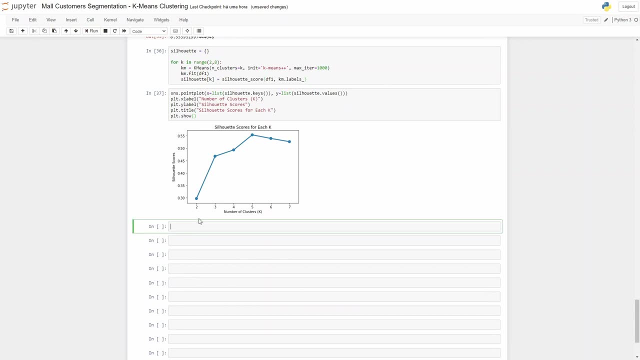 the best key. Now let's do a fast k-means So I can show you how can we plot a 3D visualization to see several features instead of only two. So for that, let's use the client segmentation, Let's use nodes. 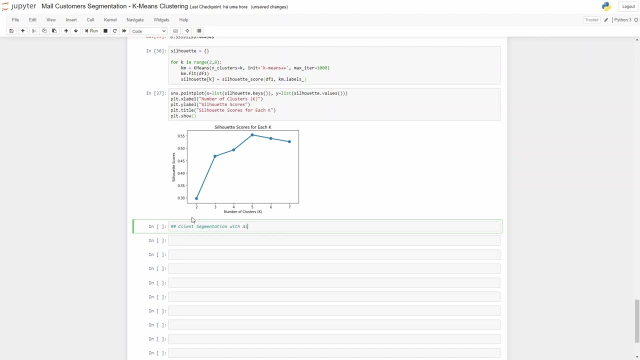 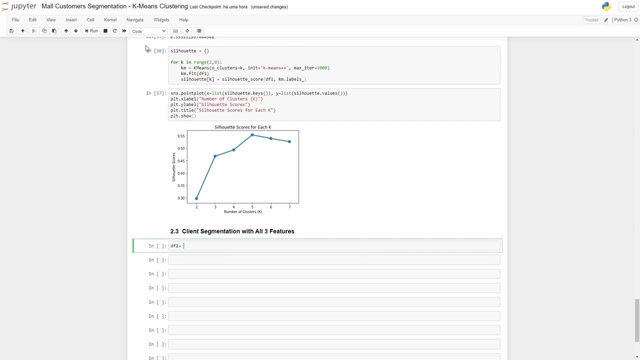 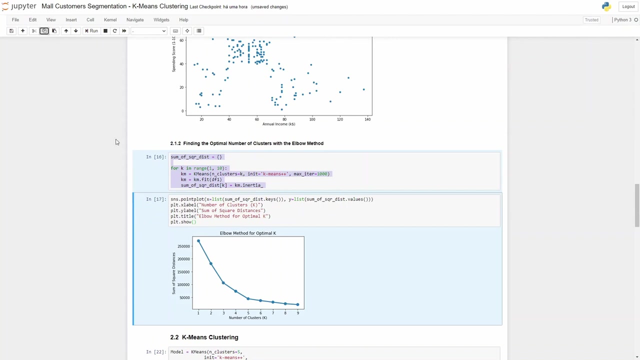 Let's build with all the three features And now we need to define the DSM. So df2 equals to dfcopy and we have our data frame here And now let's do the same as we did here: Let's find out if there is any difference between the number of k. 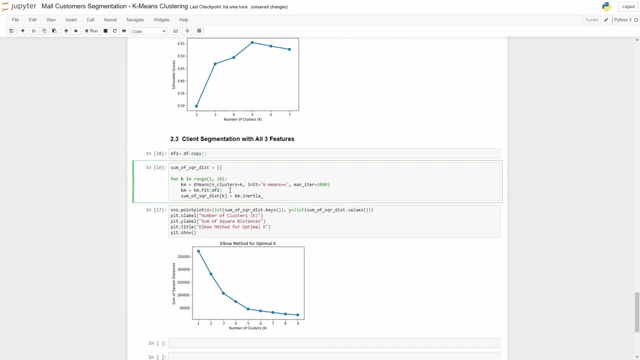 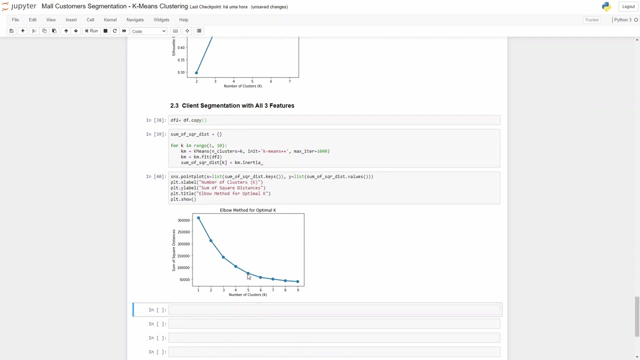 And now we need to change this to df2 and it's pretty much the same thing. Yeah, I think it's 5, 6, yeah, from 5 to 6.. Let's try 6 this time, just to see different, Because you need to choose the elbow where the inertia stops decreasing significantly. 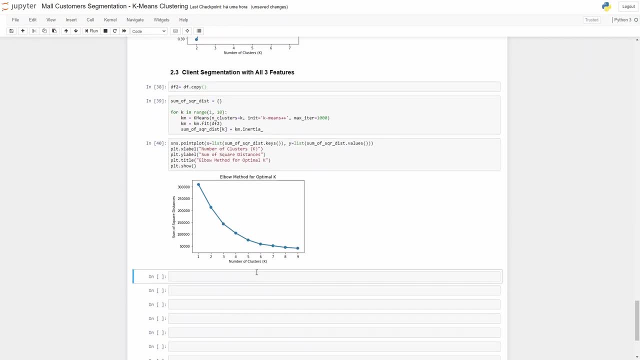 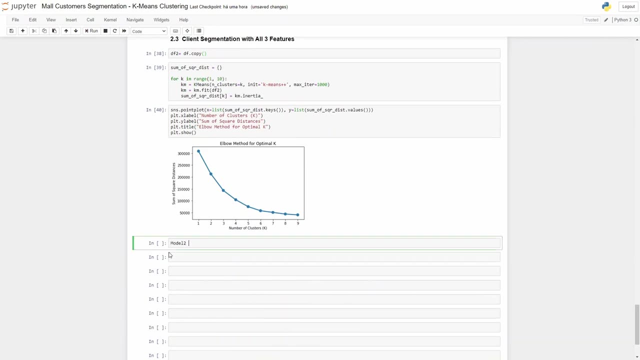 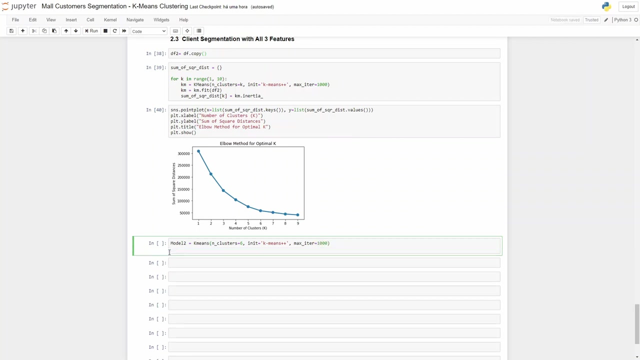 So yeah. So, as you see, it is a relative choice. So let's build the model 2.. Equals to k-means and clusters equals to 6. then init equals to k-means, plus plus again Iteration equals to 1000.. 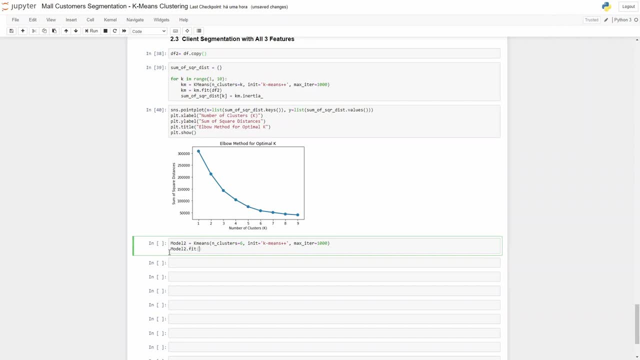 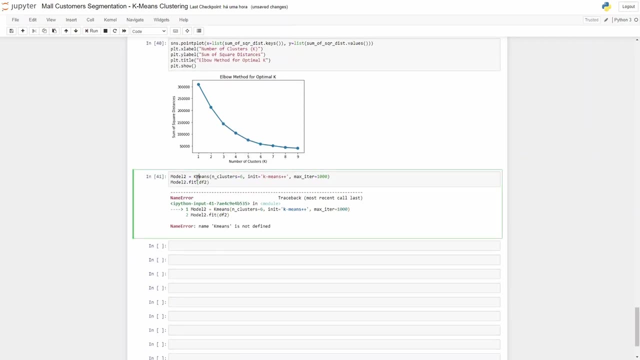 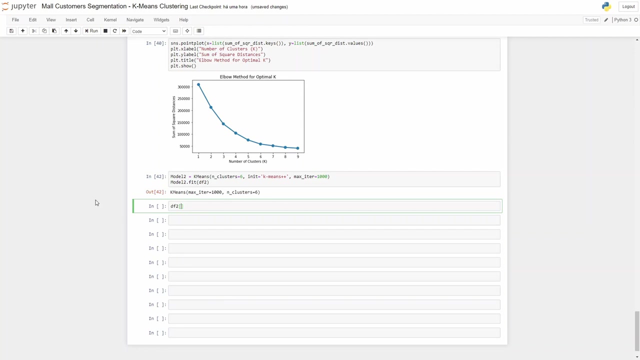 And then model 2.fit- df2.. Okay, again, Let's do it. Let's do it, Dude, I don't know what's happening today. Okay, now we need to compute or create the column for the cluster, and then model2.fitpredict. 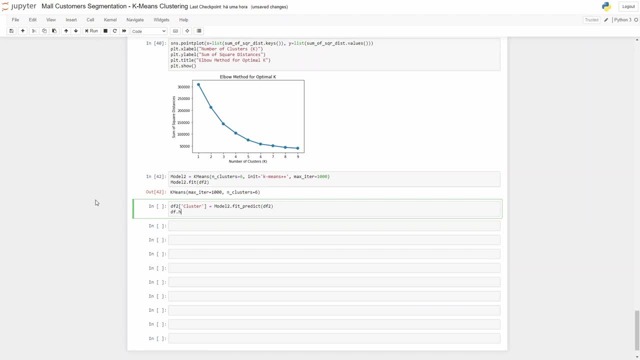 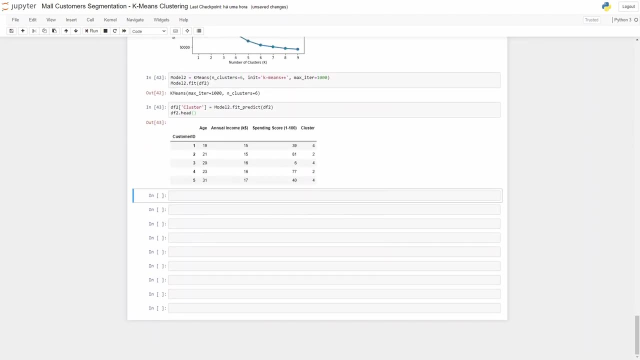 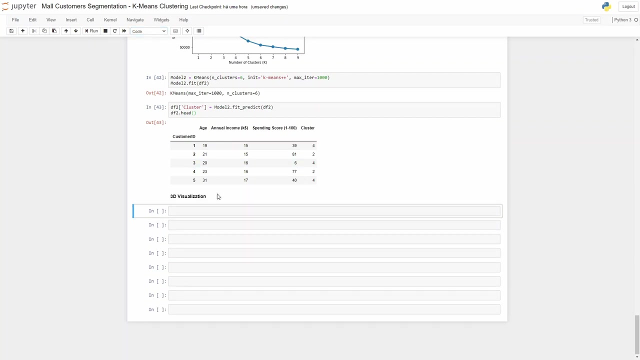 df2.. And then let's see how the dataset is Okay. Okay, Let's do it. Let's do it. Okay, That's fine, It is okay. And let's compute the 3D visualization. Let's start by defining the labels for this model. 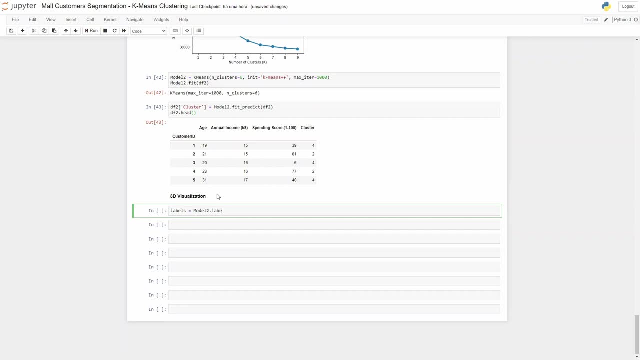 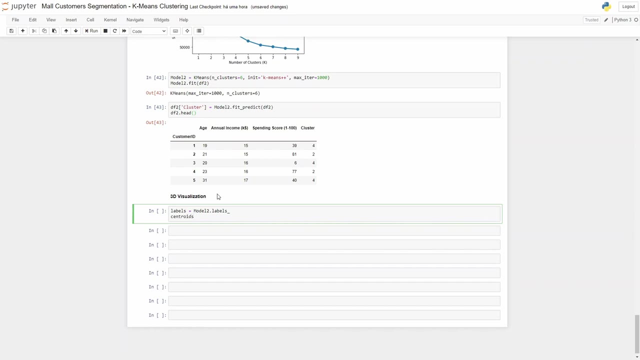 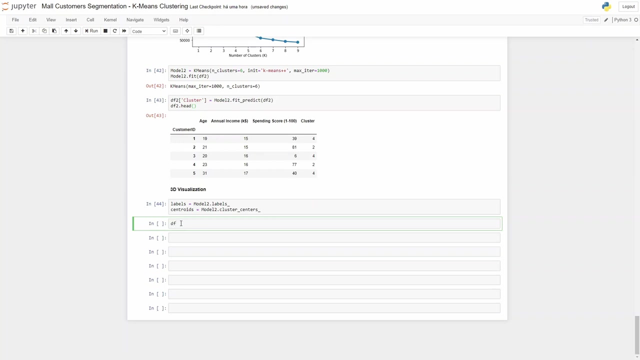 Model2.labels: Yeah, Okay, Yeah. dot labels, underscore, and now the centroid dot cluster centers: yeah, so, let's start with defining our df2 labels, which is equals to our labels, and then I set a trace and call the go dot scatter. 3d is our 3d graph. and now 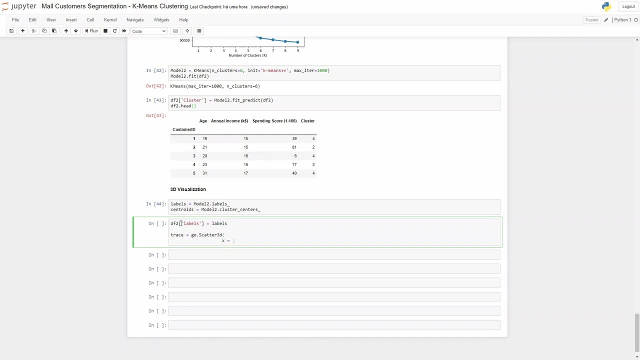 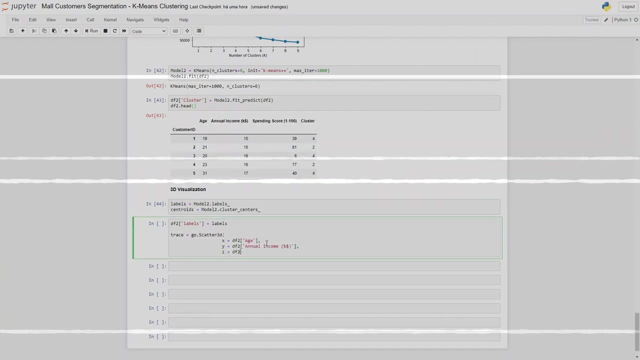 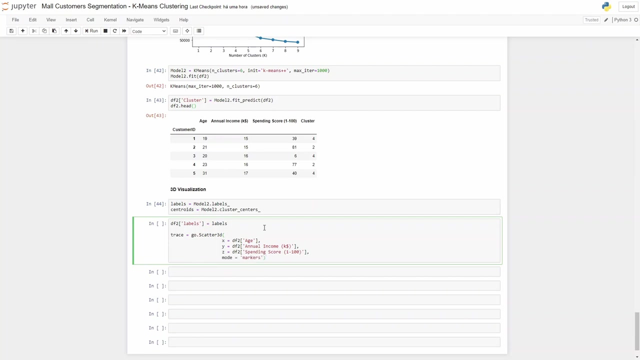 let's say that X is assigned to DF page. we need to set each one of it, X, Y and Z. and now let's set up the markers, which will be a dictionary with color equals to their assigned to the DF label. we'll define the color. next we can find the size. take us to, let's say, five, and 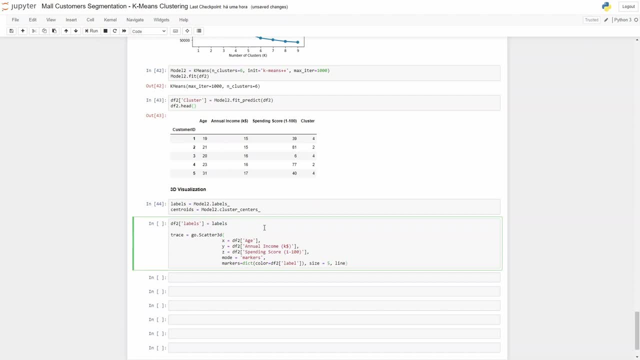 then let's define a line which is also close to a dictionary of color assigned to the df2 label: white, white, set to 20. we can even define also an opacity, for, in order to be able to see overlaps between instance, which is useful when you have a lot of data points, I can close this. 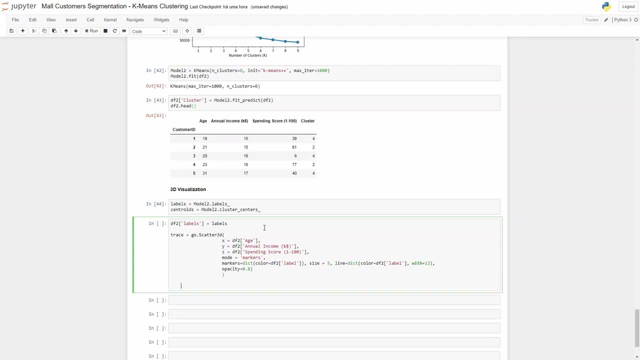 now our data. it should be assigned to the trace. and now the layout will use again: go layout title assign to website clusters and then a scene which will be assigned to another dictionary. a lot of dictionaries here, for the x-axis, which is assigned to the dictionary of 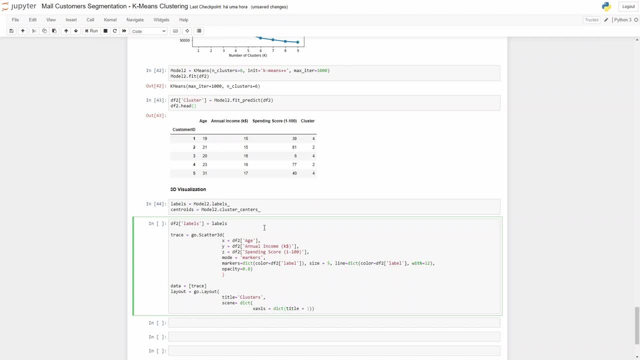 title, because two age. and now another 12 for the y axis, the dictionary with a title and erotic income, and another one for the axis with the dictionary for the title assigned to the spending score. okay, I think we are ready to finish this, and now our figure will be a code dot figure with data. 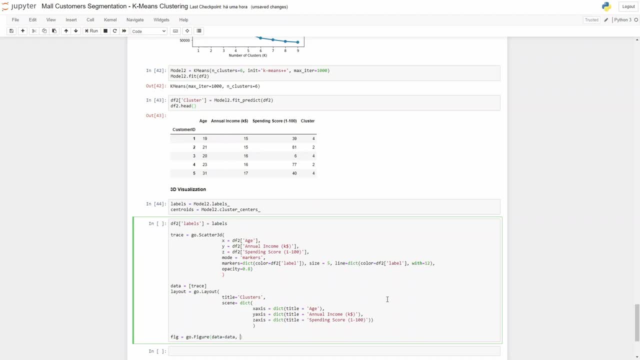 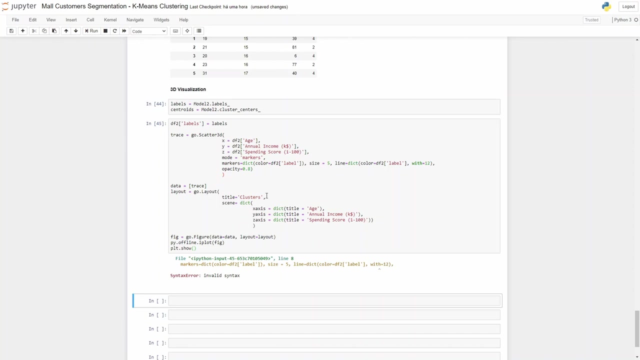 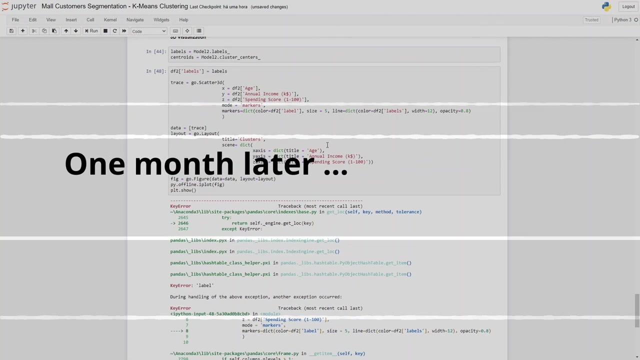 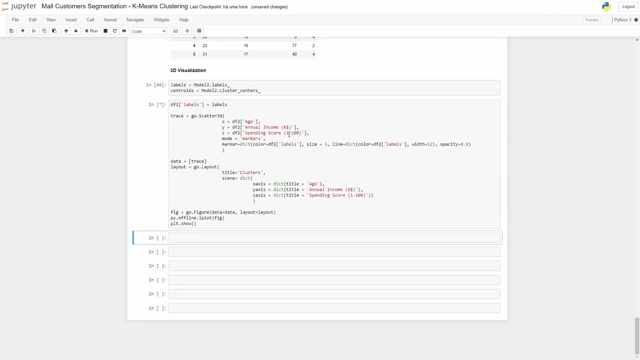 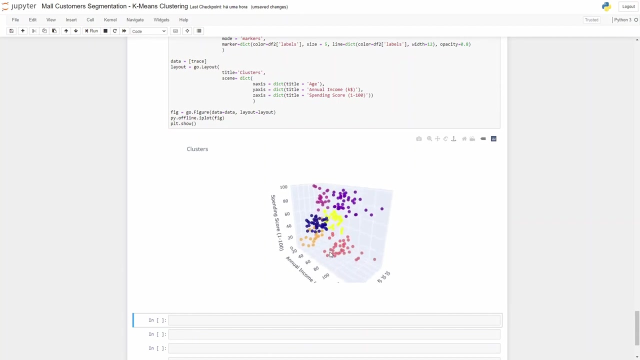 equals to the data that we define and a layout assigned to the layout that we define. now by dot, offline dot. I plot fig and now plt show and I think I'm ready. white is missing a d. this marker not markers. okay, and voila, this is our 3d plot, and here we can see clearly that. 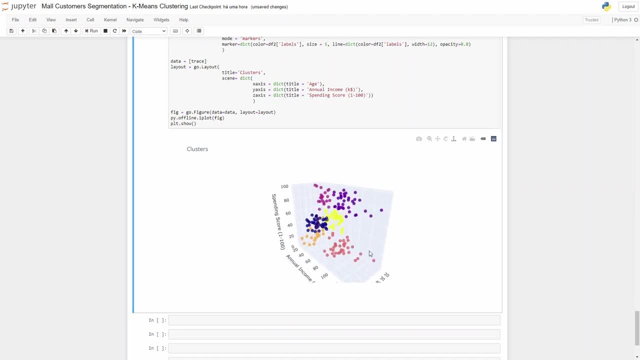 our data is divided into clusters within three dimension, so you can see it's fitted by age, we can see it's splitted by annual income and also spending score, and this type of graphs or plots are very useful to understand better the clusters when we have more than two features. 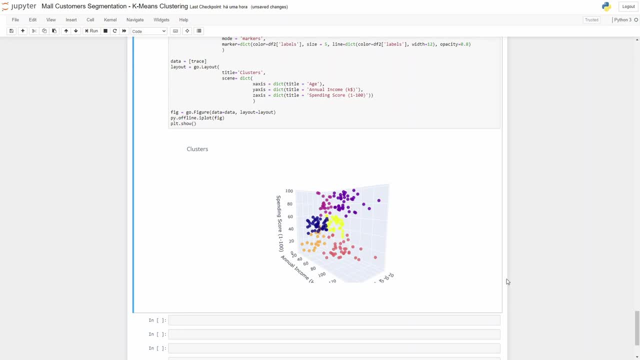 so, as a challenge, if you are doing this project, try to compute the silhouette score for each K and make a plot to visualize if the K equals to six was the best choice and, if you want, you can also use the k-means to segment the mall customers.